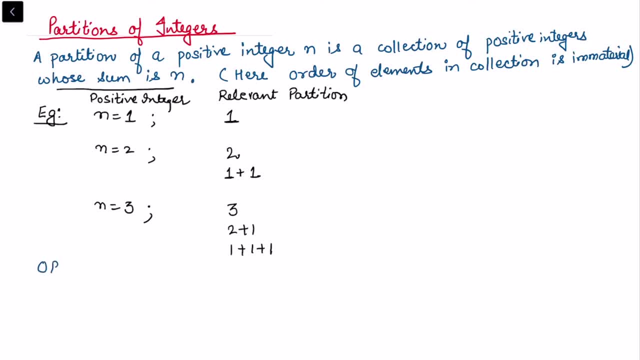 definition of the partition. so we can redefine the definition as: or partition of a positive integer. n is a finite, non-increasing sequence: n1, n2 up till nr, and these n? i are called the parts or the summands, such that if i sum these parts i get back as n, so we can even look at the definition. 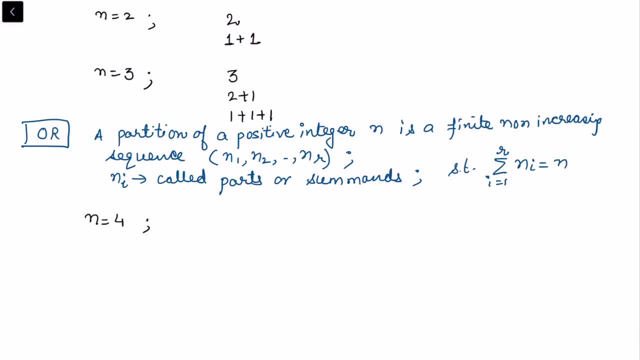 and so, in the same way i'm writing the notation for n equal to 4, so suppose, in this non-increasing sequence, what i can say, a relevant partition for n is equal to 4. i can write this as in terms of this: 4, 4. 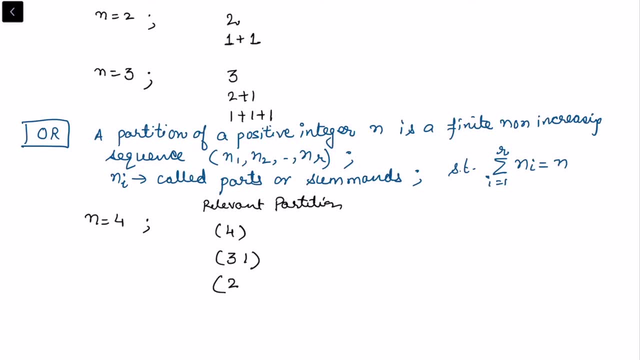 is equal to 4, or we can write it like 3: 1. so i'm writing this in non-increasing order. the parts follow the order. n1 is greater than or equal to, n2 is greater than or equal to, up till greater than or equal to nr, and these are called parts. these are also called summands in that particular. 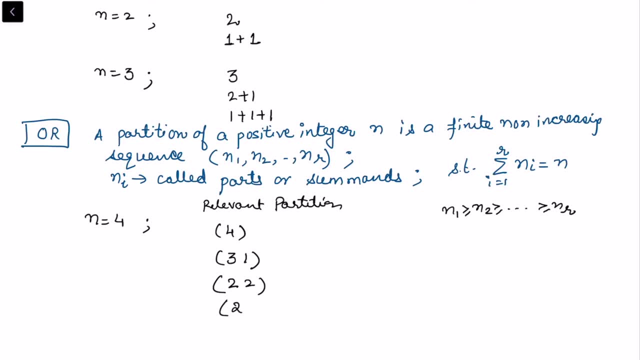 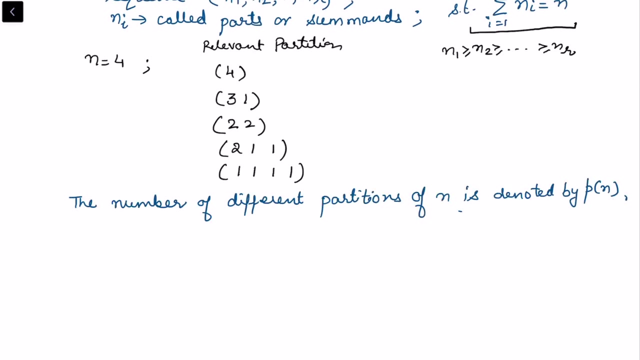 partition, we can also have the partition 2 1 1, and then we can have 1 1, 1, 1. so there are 5 partitions of 4 and such that if you sum these parts we get back the positive integer n, and the number of different partitions of n is denoted by pn. so in this notation, if i want to, 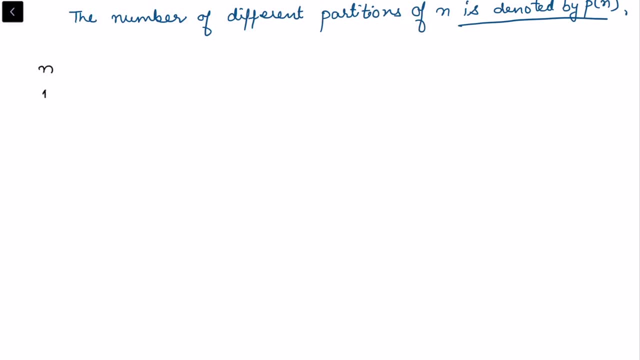 rewrite this whole table. we can write n, 1, 2, 3, 4, 5. that i've already written. suppose this is the positive integer, and here i want to write all the relevant partitions of n, as i've just explained. 1 has only one partition, 2 has 2, and then 1 plus 1, 3 has 2, 2 plus 1, and then we got 1 plus 1 plus 1. 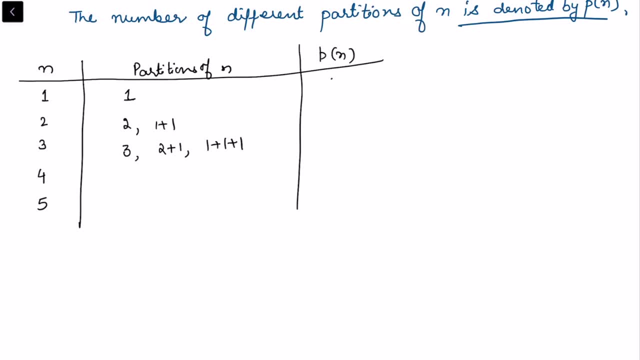 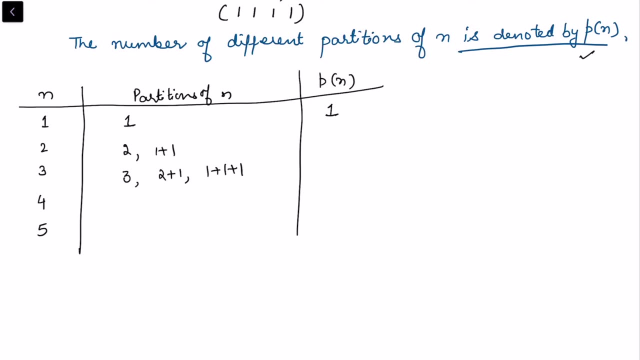 so, correspondingly, what is the number pn? pn is the total number of the partition and which we denoted by pn. so in this case, n is equal to 1, there are 1 partition. when n is equal to 2, there are 2 partition when 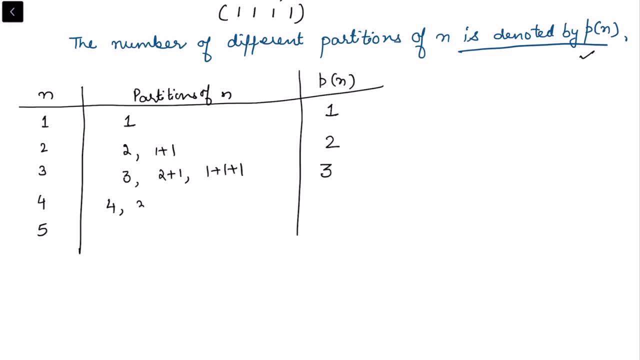 n is equal to 3, there are 3 partition for 4. we got 4, 3 plus 1, 2 plus 2, 2 plus 1 plus 1, and then 1 plus 1 plus 1 plus 1, so there are 5 partition and for 5 there are 7 partition. for 6 there are: 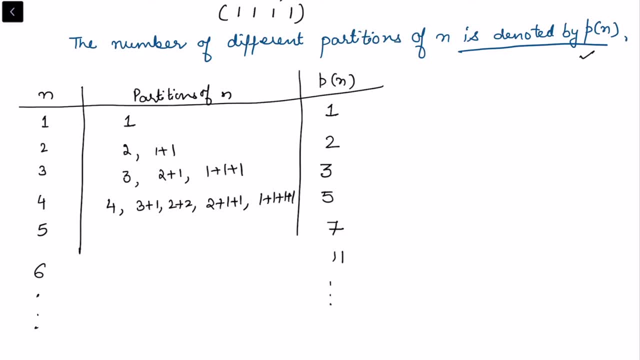 11 partitions and we can continue this table for 5. i'll write also so for 5 we can see there will be a 5. then we have 4 plus 1, then we have 3 plus 2. we can have 3 plus 1 plus 1. we can have 2 plus. 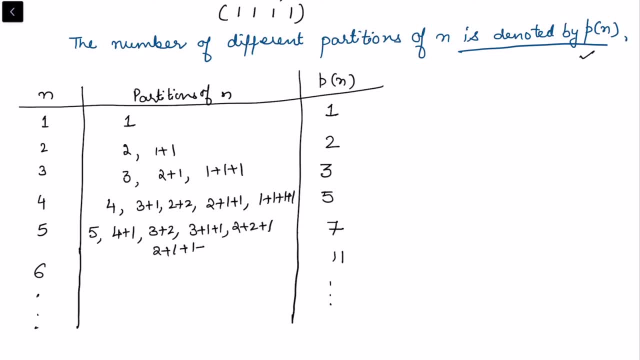 2 plus 1, or we can have 2 plus 1 plus 1 plus 1, and then we can have 1 written 5 times. so these are the relevant partitions corresponding to 5. we can even write- we also note here, note 2 plus 1. 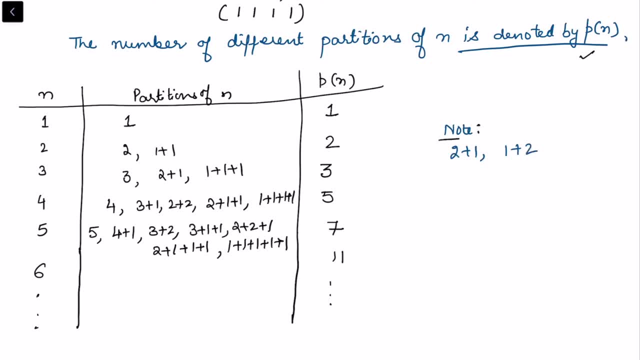 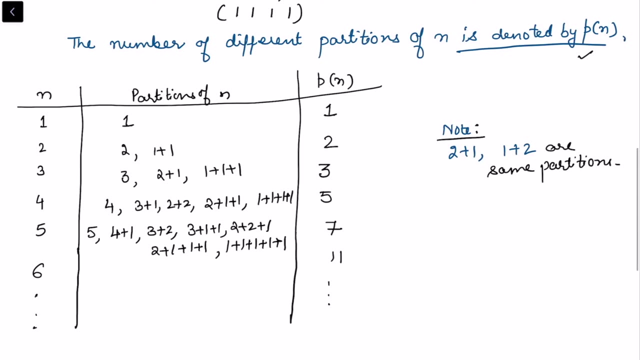 and 1 plus 2. these are. these are same partition. we have already written that the order is immaterial, so this is already written in the first definition. ordering is not matter. so in case we are considering an ordered partition, that is called as a composition. so currently these are same. 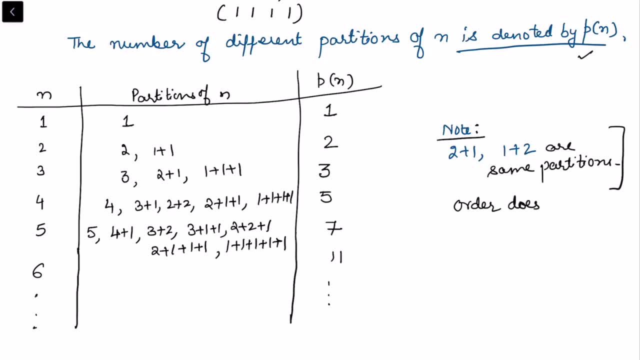 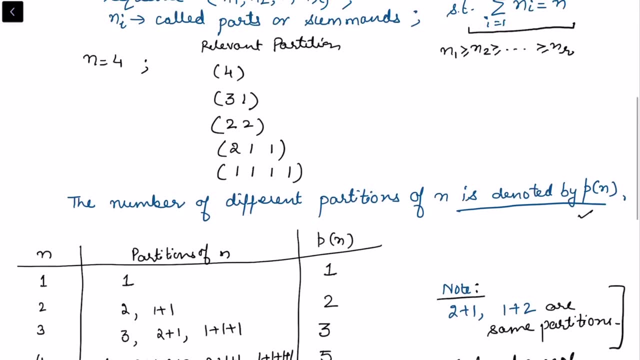 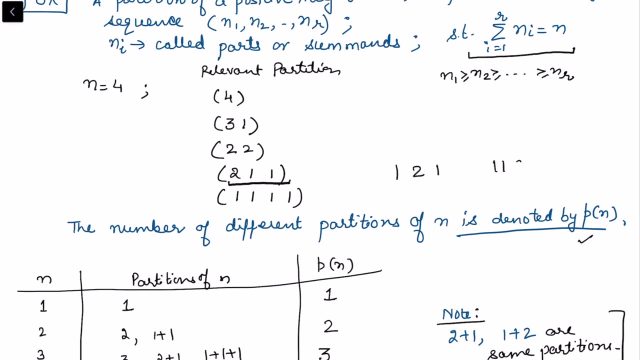 partition and we say order does not matter. so just to be brief, that we do not get confused in the order we define, write the partition in a non-increasing order so that we always write like 2 1, 1 and we do not get confused in 1 2, 1 or 1 1, 2, they are same. 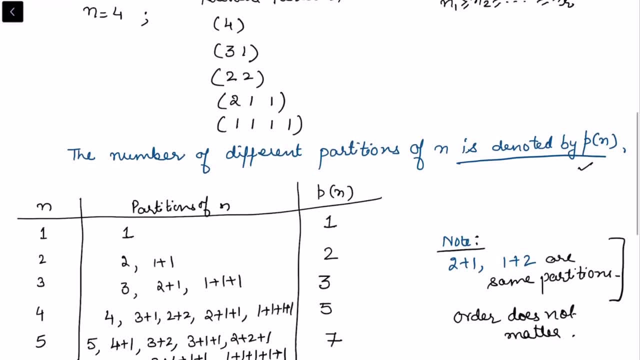 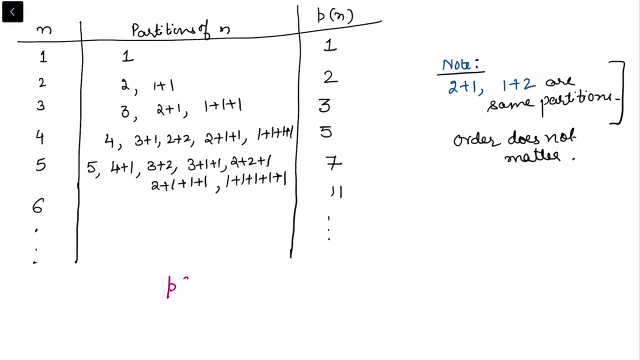 so this is why we have mentioned clearly that order does not matter. now the question is: how do we generate this number, pn? what is the exact formula for pn? or is there any generating function corresponding to the pn for which we can know? if i want to know what is the partitions corresponding? 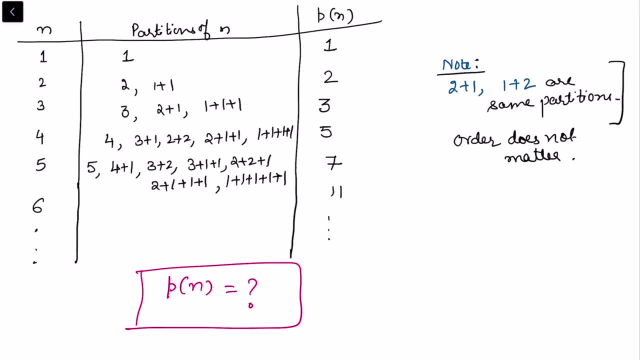 to n is equal to 10, or for corresponding n equal to 100 and so on. how do i find this number pn? because it will be difficult to write manually all the partition and this number goes very, very large. so we will look this problem using the generating. 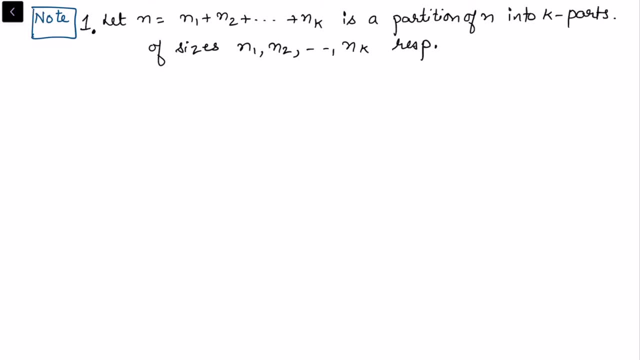 function. so we look at some more nodes in this partition. let n is equal to n 1 plus n 2 plus n k and if you notice that we have taken in this is a partition of n into k part. so this is what we mean and the parts values are different. so when we say part value, we do not call this as a value. we 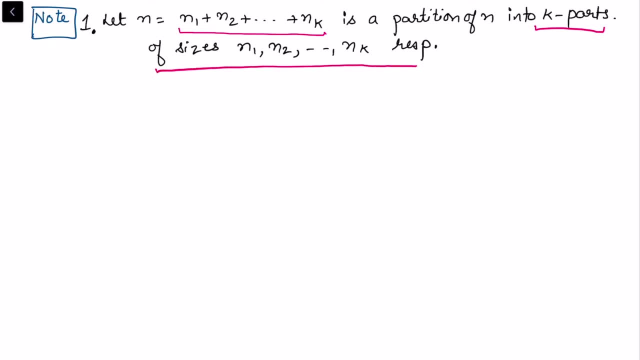 the part has size n1, n2 up till nk respectively. so for this you can consider an example. say for example, i take n is equal to 5 and i want to write partitions of 5, so we can say partitions of 5 into 3 parts. so suppose i want to write like this one into 3 parts of size 1 and 2 of sizes. 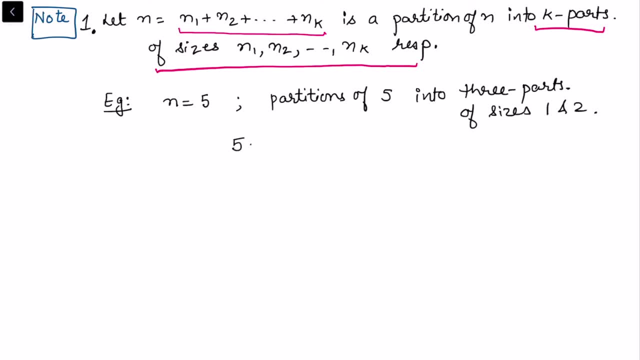 1 and 2, so i can always write 5 as 2 plus 2 plus 1 here. this is the value for n1, this is the value for n2 and this is the value for n3. remember, in the definition we have said n1 is greater than. 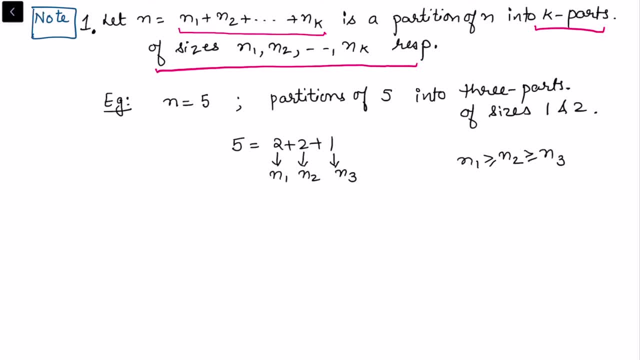 equal to n2, is greater than or equal to n3. so the strict inequality is not there. we can always take the part size as equal. we can see one more example. suppose, consider, n is equal to 9 and i want to write the partition of 9. so 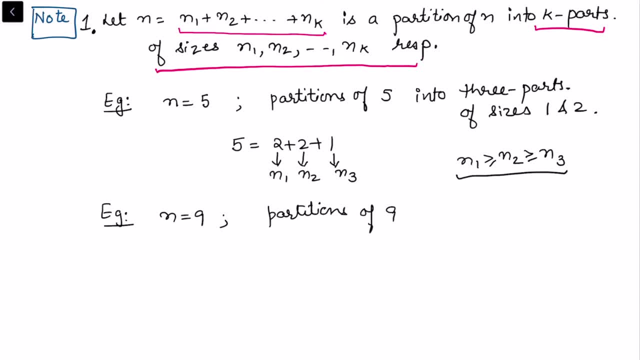 so if i just consider partition of 9 into 4 parts, and these parts i've considered of sizes 3, 2 and 1, so i want to create a partition of 9 with these three sizes. that means 3 plus 3 plus 2 plus 1. now 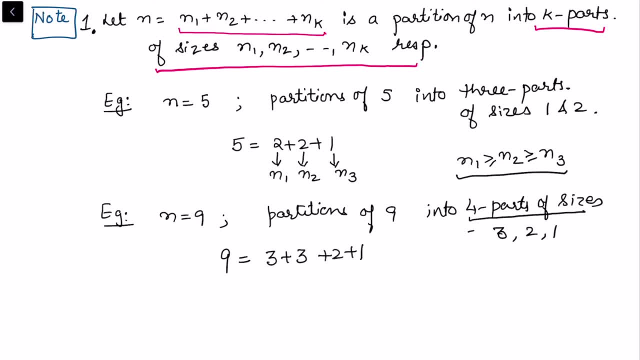 when you say the partition of 4 parts of size, you can even write this as 3 comma 3 comma, 2 comma 1. so it just depends upon how do you have written. so here i've said that the part sizes are actually coming from. 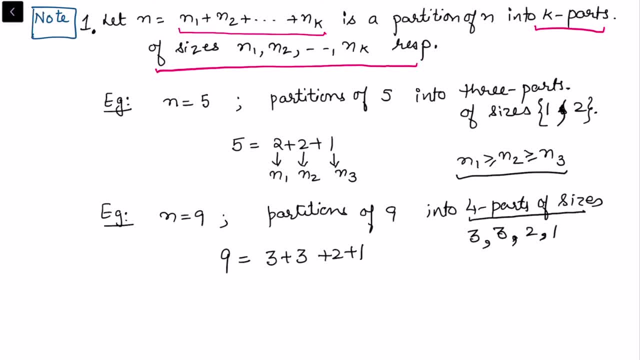 the set 1 comma 2. this is what i mean. so when you specifically give the value for the part sizes, then also you can directly use them: 3 plus 3 plus 2 plus 1. so these are just the male, the symbol or the notation, how you want to define the set, whether you want to give every uh value for n1 and 2 and 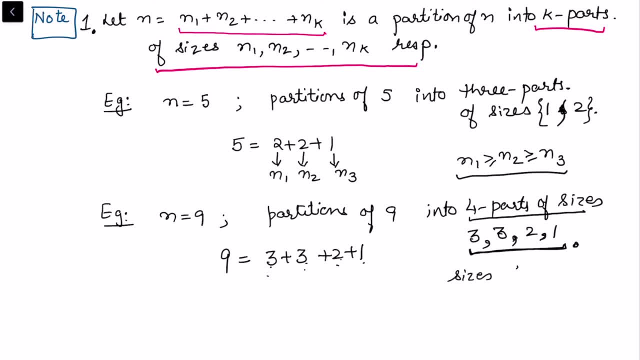 3 and 4, or you can say the part sizes are belonging to the set 1, 2 and 3, and then you can create a partition of 9 from that. so this way we know now the notation of the length of the partition and we can also say length of partition. length means how many parts are there and that 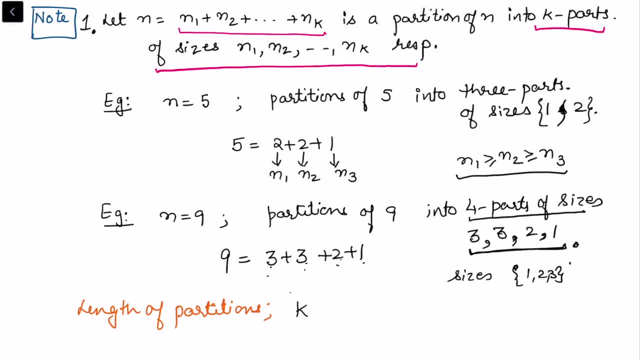 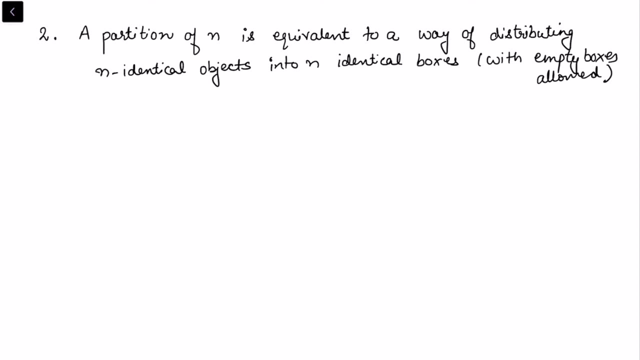 length of the partition. you is here as k because you can see that we have used k parts in a particular partition. so we have a concept of the length of a partition, into how many parts and what are the sizes corresponding to each part. now in this note i can consider a partition of n. 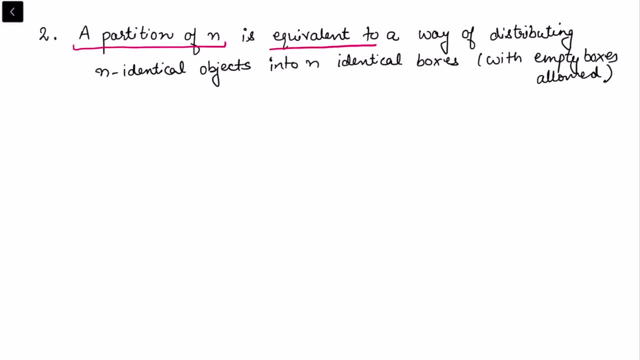 is equivalent to a way of distributing of n identical objects into n identical boxes, with empty box allowed. so we can always see a partition as a distribution problem. and in this distribution problem let me to take an example again, for n is equal to 4 to explain this problem. so suppose that 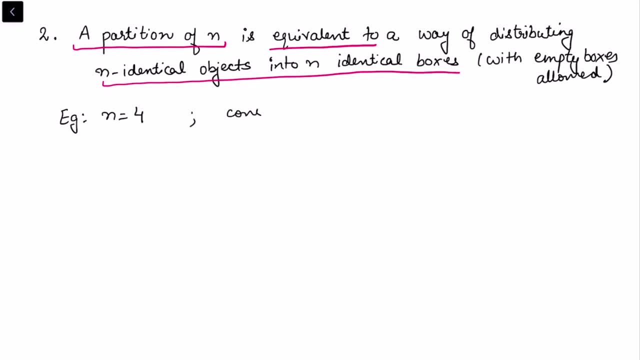 we have n is equal to 4 and consider 4 boxes. so we just consider 4 boxes. okay, so we have total n as an object. so this is the n equal to 4 and we just consider the same number of identical object. so suppose i consider 4 boxes and we just show. 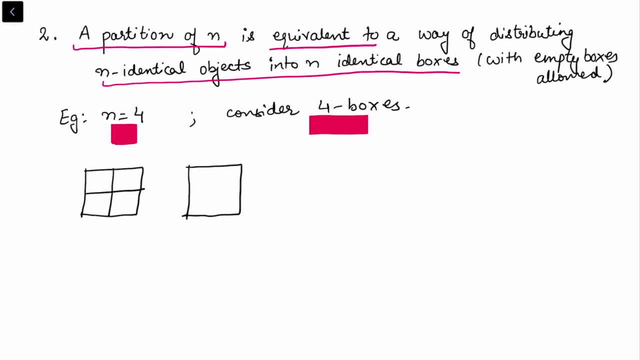 them like this one. these are the 4 boxes and we just need to know how many partitions are there. 4 has 5 partition, as we have already explained. now, what were the partition for 4? the first partition for 4 was 4 and 4 has 5 partition. so we have 4 boxes and we just consider 4 boxes and 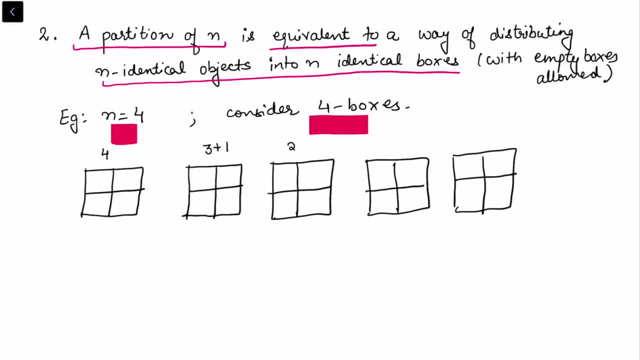 4. the second one was 3 plus 1, and then we have 2 plus 2, and then we have 2 plus 1 plus 1, and then we have 1 plus 1 plus 1 plus 1. this is what it means now. if a part is of size n equal to 4, that means 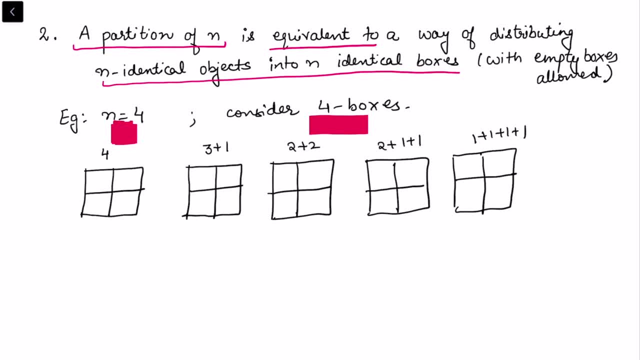 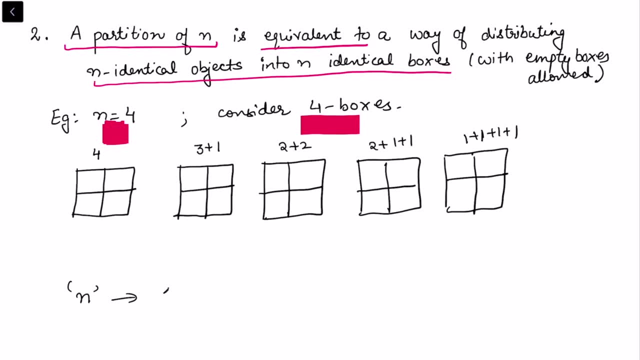 the maximum box that we can allow is 4, because the least value for the part is 1. so if you take any number n, the one of the corresponding partition is 1 plus 1 plus 1, repeating n times. so this is what it means: a part of size n can go in maximum n boxes, and that's how we are trying to. 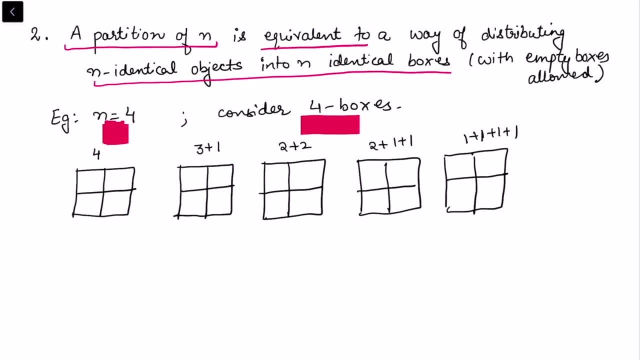 relate this distribution problem of n identical objects into n identical boxes. so in case this value 4 is there, we'll assign one box with all the 4 object, and here we are only using part as 1. so there is only one part in the partition. there are two parts in the partition, 3 and 1. 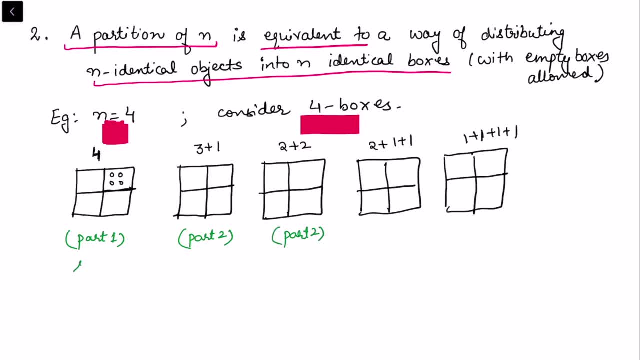 there are two parts in the partition. here the size of the part is 4. here the sizes are different, so we have two sizes, 1 and 3. here the sizes are same, so we have 2 and 2. either you can simply write as a set notation 2 or you can say that we have two sizes, 2 and 2, with with the two parts. 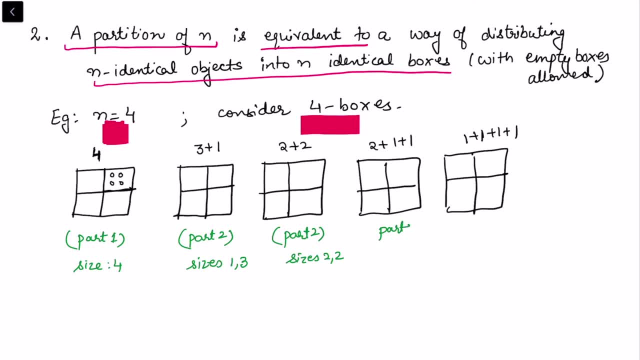 here there are. this is a partition into three parts, so we got three parts and here the sizes that we have used is 1 and 2, one, one and two. and then we have- this is a partition into four parts and we used only the sizes one, one, one, one, or we can see we use the sizes belonging to the set of one, so we can. 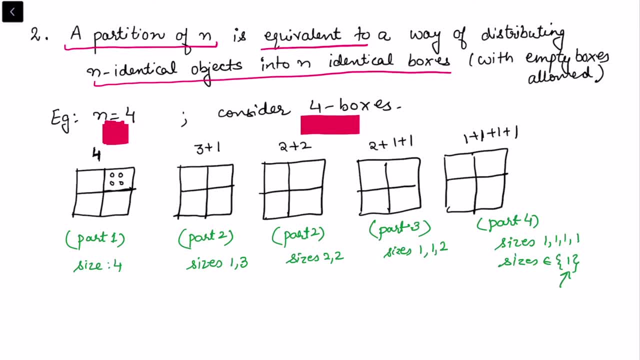 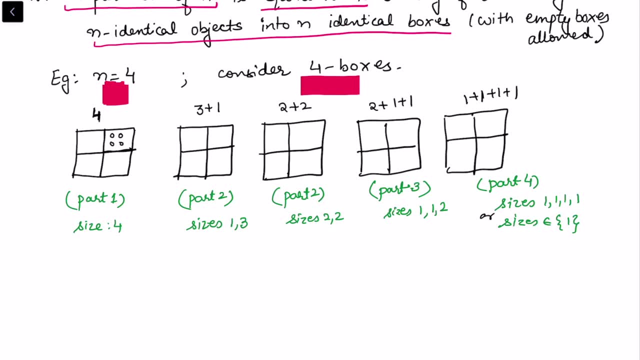 only use one as a partition, or any partition which is constructed from this part size one. so this is what do we mean now? how do we distribute, as in case of the first i've shown, since there is only one box, part one, that means only one box and we place the size, so there are. 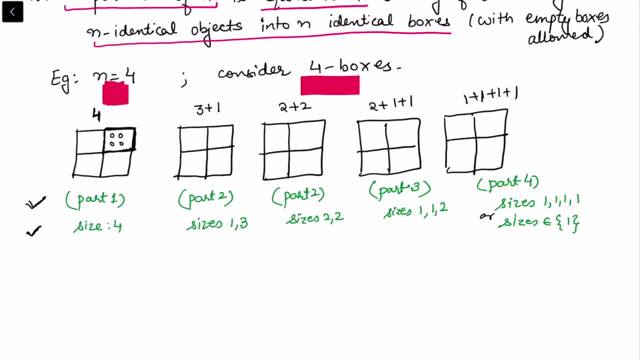 four dots or four zeros. that i've shown. that i've shown here to show the partition of size four. now three plus one. there are two parts. that means i'm going to use two boxes. in one box the size is one and in another box the size is three. you can place it anywhere, three or one. order is the. 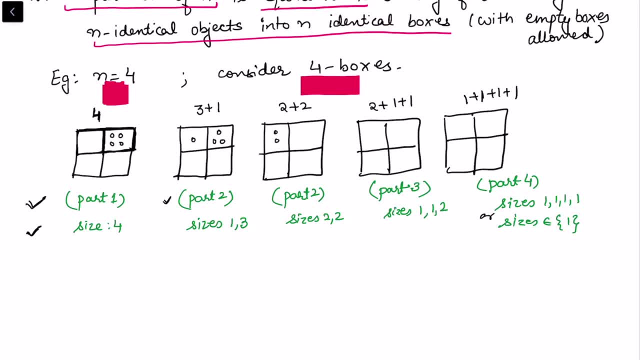 material. then in one box we have two and in the another one, also we have two. we can use two boxes because of the part as two. then we have part three, and in this case we can use two, then one and then one, and now, for this case, we will have one, one, one, one, one, one in each one of them. so now, as we know, the number p? n this: 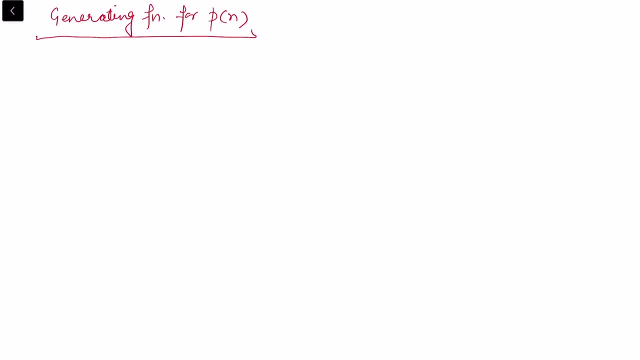 is equivalent to the number of ways in which our identical objects are distributed amongst n identical boxes. so we definitely want to know what. how do we calculate that count rather than making separate cases, as i've explained for the example, for the case n is equal to four, what would be in general for any n. so this means we. 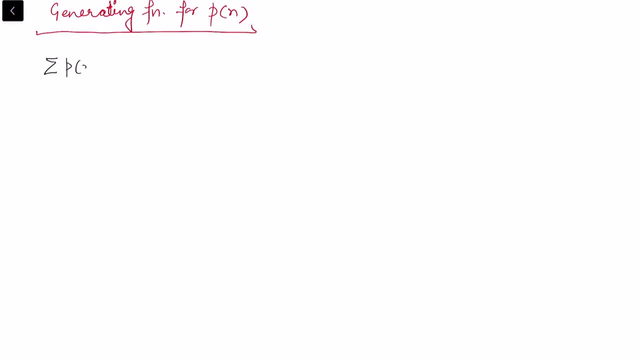 must need to understand what is the generating function for p n. so p n, that is the number of partition of n integer into x to the power n, and varies from zero to infinity. and on this side, now notice that for this n integer, this is the positive integer for which i'm seeking to write. 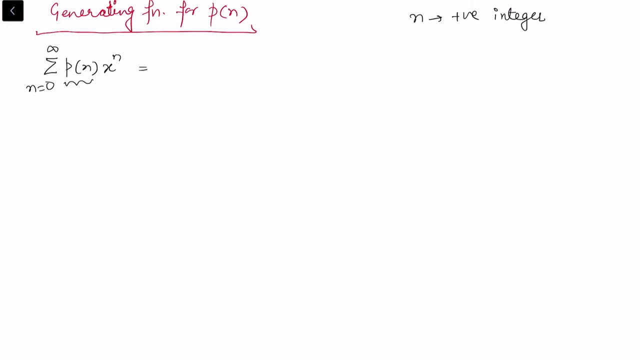 all the partition and here there is no restriction on the part size. so we can say no restriction on, no restriction on part size, so any part size may, can come. we have seen in the definition a positive integer and has a partition into positive integer, so the positive integer starts from. 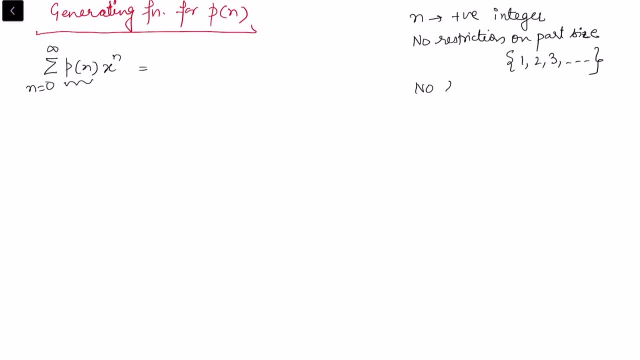 1, 2, 3 onwards, and then there is no restriction on the length of the partition. so on partition, so no restriction on length of partition. 미�크는 그 판 명량에서. and we have seen that there is no restriction on length of the partition. length means that 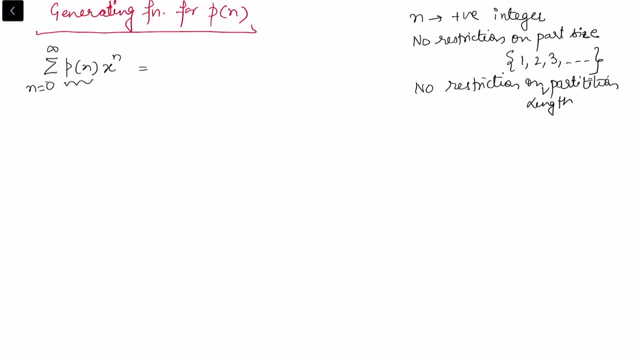 if the part size is equal, you can write the partition into two part or three part or four part and so on. so in this case we can simply write again in the similar way as we did in earlier. suppose i consider the part one, and this part can appear or it may not appear. x to the power zero, sorry. x to the power one can. 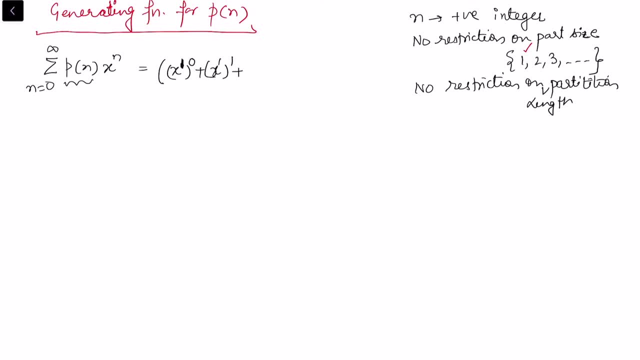 come in zero time. x to the power, one can come in one time and repeat repetition. then the second part: x square, this can come zero time. x square can come one time, and so on, and we continue this process. so we see that this is same as one plus x to the power, one plus x square, and so on, and 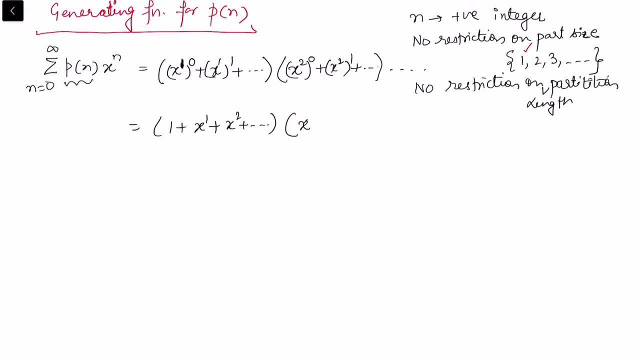 then, if i just look at this one, this will be again, the first term will again be one, then we will have x square, then we will have x to the power four, and so on, and we will have the remaining term, x, three, and then x to the power six, and so on and all the terms. so, because there is no restriction, 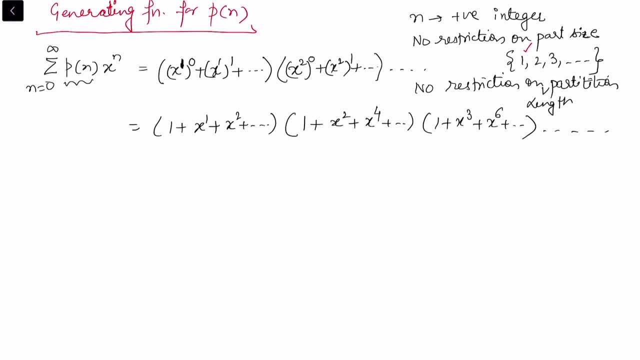 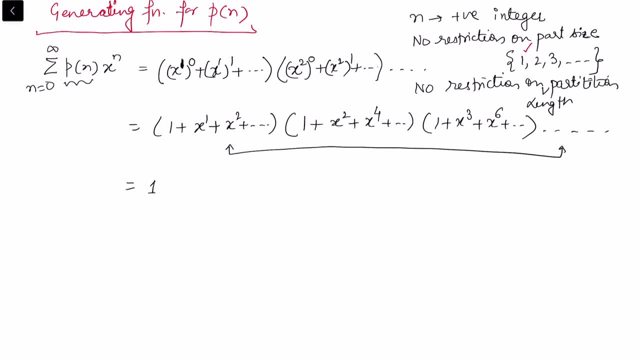 to understand. what do we get? we will get here. the constant term will multiply 1, 1, 1. when we multiply this, we get 1, and then we will get a coefficient of x to the power 1, which will be 1. 1 can verify by simply multiplying. we will see 2 x square, then we will see 3 x cube, then we will. 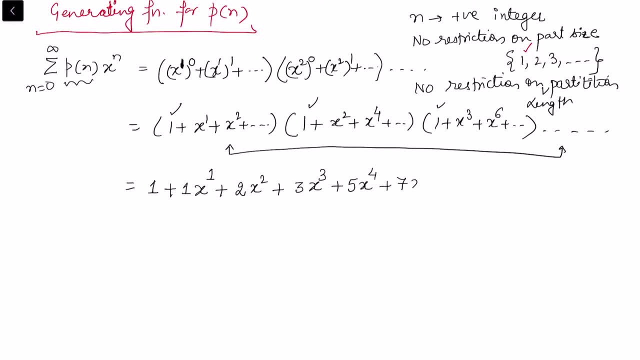 find 5 x to the power 4, and then we will have 7 x to the power 5, and we will have 11 x to the power 6, plus so on. now this means this is the partition of 0. p. 0 is equal to 1. this is by convention, that 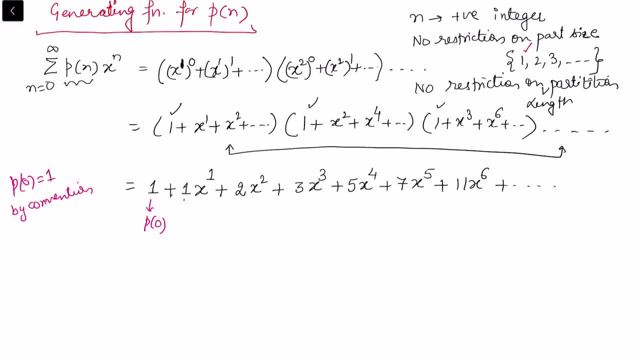 the 0 has a partition as 1. this is the partition of 1, because x raised power 1, which means that the coefficient of x raised power n gives the partition of n. this is the partition for 2. this is the partition for 3. this: 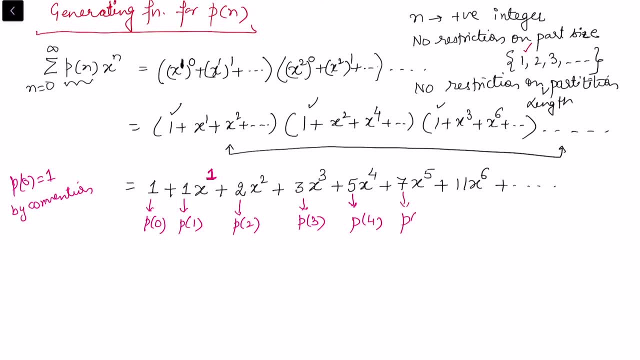 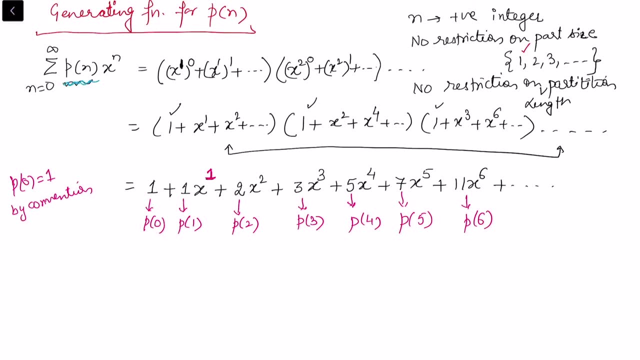 is the partition for 2, this is the partition for 3, this is the partition for 2, this is the partition, is the partition of 4 and this is the partition of 5, this is the partition of 6 and we continue. that is why we have written on the left hand side, p and x to the power n, now in terms of the closed. 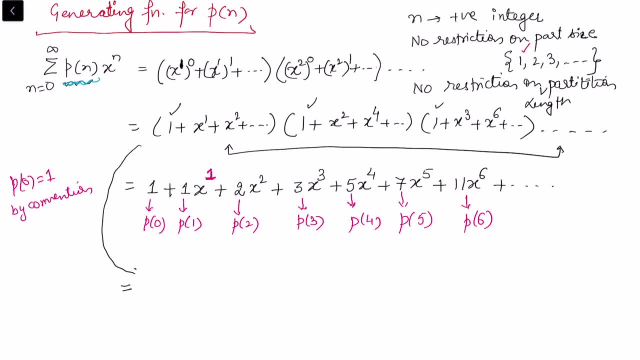 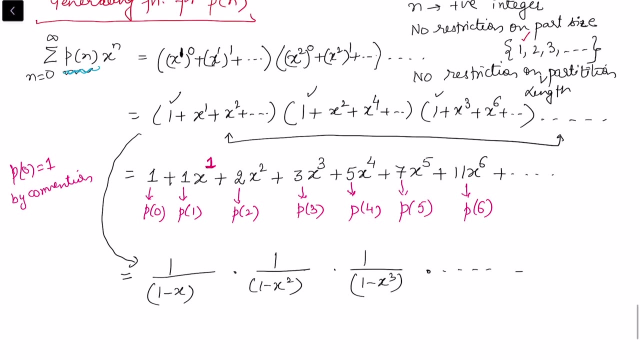 form. if i just look at the first expression, now this is like a gp, and so we can write it as 1 over 1 minus x, similarly the next term. i can write 1 over 1 minus x square, similarly the next term, 1 over 1 minus x cube, and continue the product. so now this is same as product. so this is the symbol. 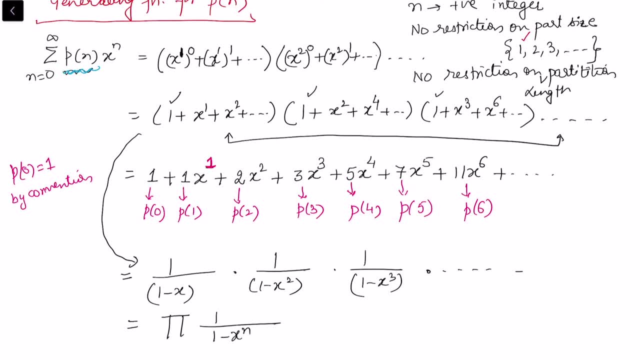 for product 1 over 1 minus x, to the power n, n varying from 1 to infinity, and this becomes the generating function for partitions of n. so if you want to write the partition of n into any number of parts, then this becomes the generating function. so now suppose we want to understand the generating. 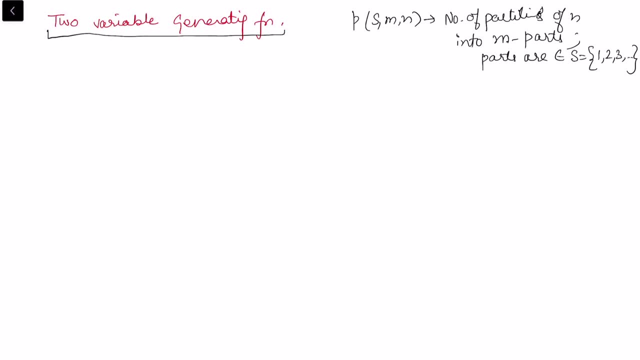 function where the partition length is fixed. suppose i want to say that we are distributing r object into two identical boxes, so the length is fixed. or maybe the r is fixed in, because in the earlier case we have considered the partition length as complete, the maximum possibility. so for example, 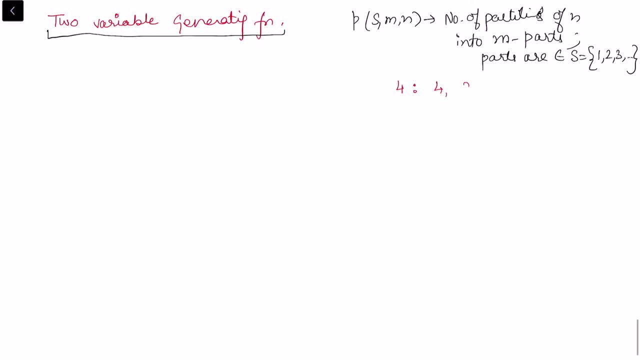 the partition for 4. we have considered 4, 3 plus 1, 2 plus 2, and then we have 2 plus 1 plus 1 and 1 plus 1 plus 1 plus 1. now suppose i just want to consider the. 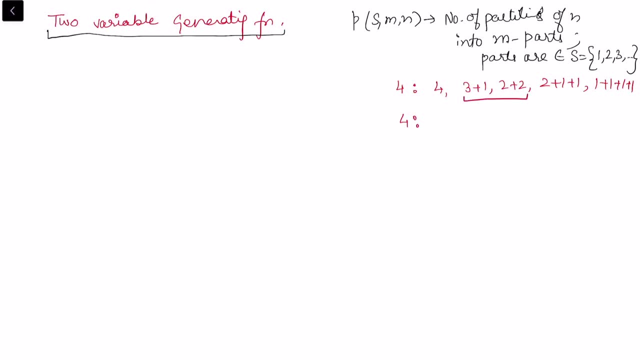 partition length as complete. so, for example, the partition length as complete. so, for example, the partition of 4 into length 2. so that means only these two, i am talking. so this way you can also extract these. there are two partition of the length 2. for this we will create a two variable. 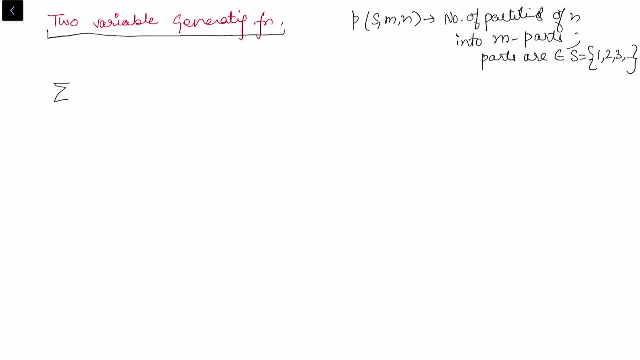 generating function, and so this will. i will not add much theory here because that will be again another understanding about two variable generating function. but just to give you an idea, let me first define the partitions z to the power m, x to the power n. this is same as product. 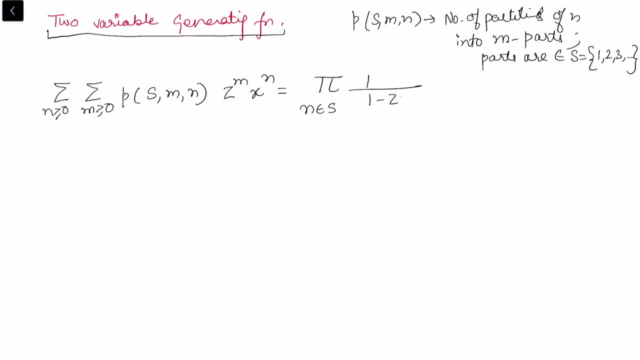 n belonging to the set s, 1 over 1 minus z, x to the power n. now this i have already defined here. p s m n means this is the number of partition of n into m parts. so m parts means that's how the length is fixed. so for example, the partition of 4. so we will say partitions of 4 into 2 parts. so 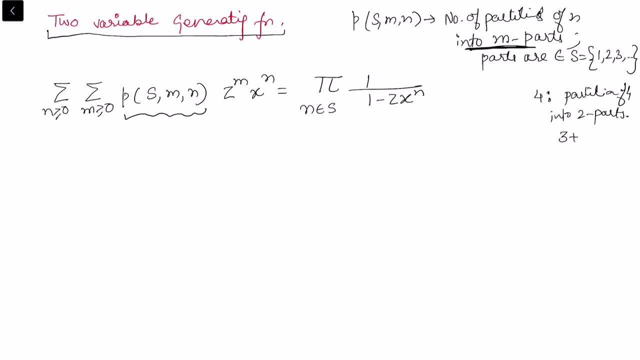 when i say into 2 parts only, this means i am writing 3 plus 1 to the power n. so this is the number of partition of 4 into 2 plus 1, and i am writing 2 plus 2 and then you can say parts. 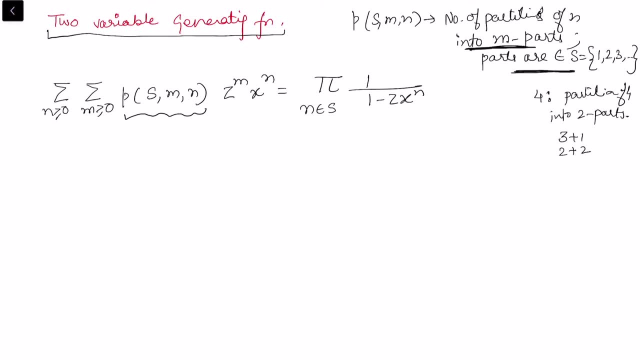 belonging to the set this, so you may further restrict the part size. so in this case we may take 1, 2, 3 and what so on. so now this is same as z to the power, m, x to the power. so you have two variables actually here, and then you can say the z raised to power 1. so this is the part size. 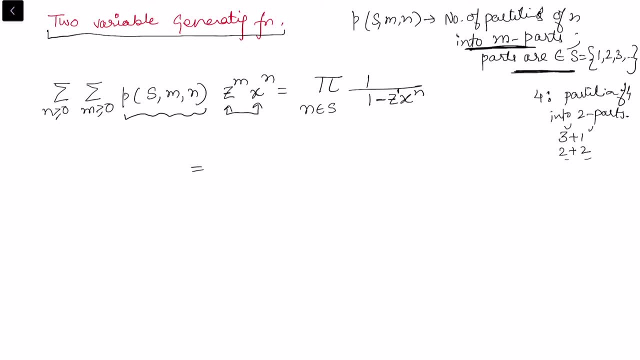 1 and then increase and then open this expansion. so when you open this expansion again you will get some expansion, something like that, the constant term. then there will be something z 1 x raised to power 1, then there will be something z z 1 x square, then there will be something z 2 x square plus so on, so something expansion like. 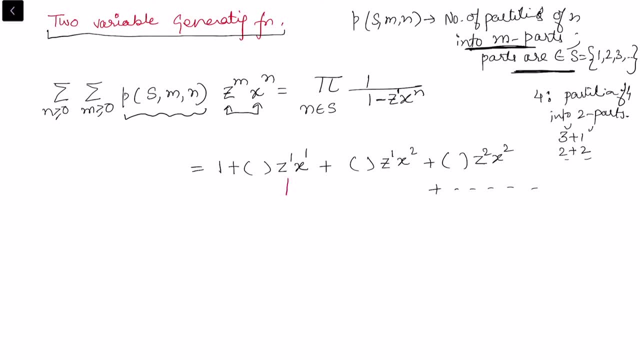 coming up this one now. how will we read? this means that because of the x power, we will say that this is a partition, of partition of 1 into 1 part, into 1 part. so z's power is going to tell me how many parts and x power will going to tell me the. 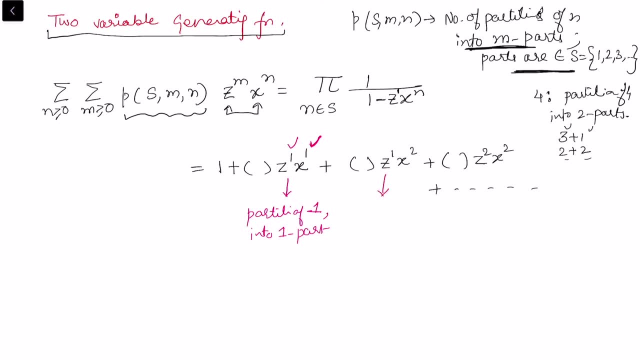 partitions for the corresponding integer. this will be telling me the partition of 2 into 1 part and in this case, when i say partition of 2 into 1 part, which will be relevant only 2. partition of 2 into 1 part is 1. here this will be only 1, so the coefficient for this, when we expand the previous. 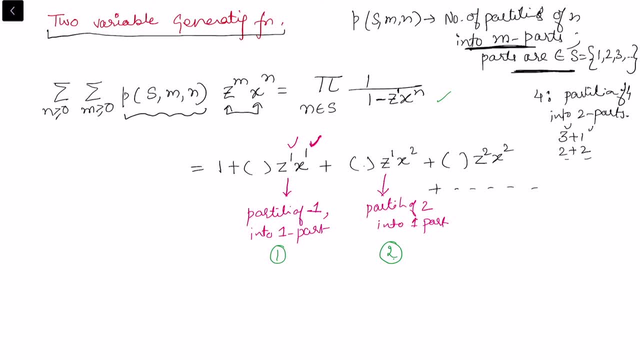 expansion will be only 1 and that 1 relevant case is 2. now, similarly for the next case, how i am going to read for this particular case. i am going to read it like this: is partition of 2 into 2 parts. so when i say partition- 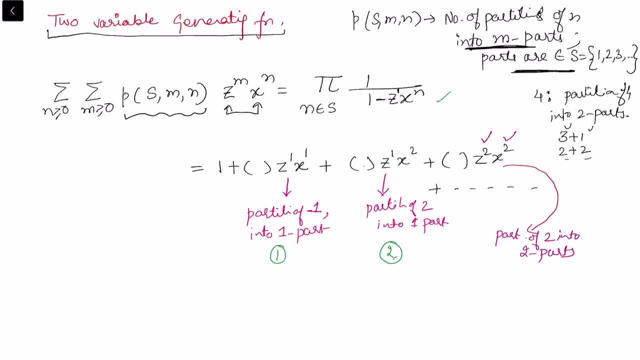 of 2 into 2 parts. this means there will be a partition of 2 into 2 parts, 1 plus 1, and that will be the relevant case and again this is equal to 1. but when we uplift the condition, say, suppose i want to now. 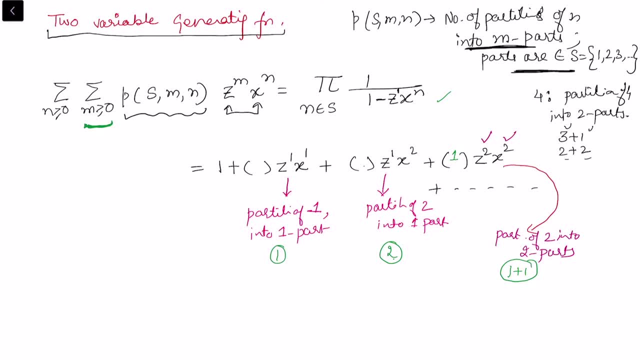 club. this m goes from 0 to infinity and i just want to reach to the previous function. so in that case you can simply put: z is equal to 1 and your case translate to the single variable generating function. so this will translate to single variable generating function and in this case you can see: 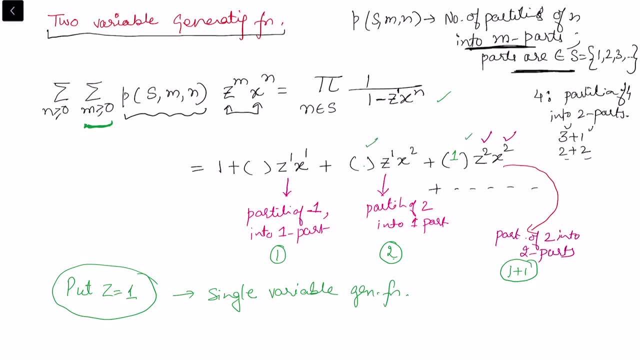 again the one relevant partition here and one relevant partition here because the both give me the coefficient of x square. they are going to add and we are going to get back to the same condition of the. there are two partition corresponding to the integer 2, so this way we can understand further the distribution. 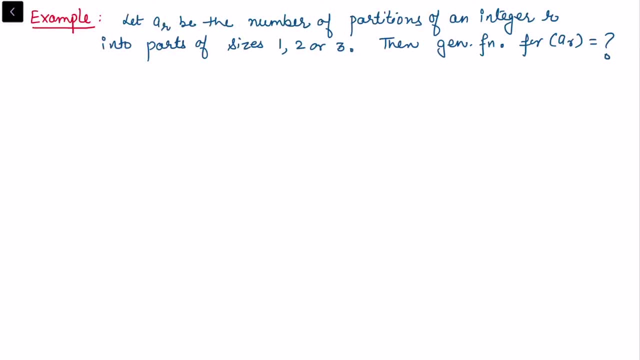 problem using the partition function. now we understand the partitions with the restricted part size in a generating function and in this question let a r be the number of partition of an integer r into parts of sizes 1, 2 or 3, so that means r can be any number it can. 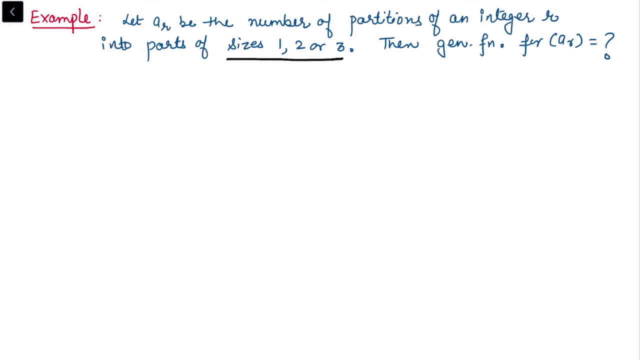 be even 1, 2, 3 or up till infinity or 100, but the only thing that i want to use the corresponding partition in terms of the size: 1, 2 or 3. so before i write the generating function, let me to just explain this problem. 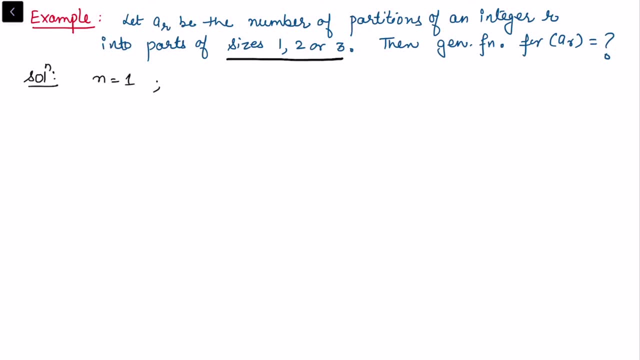 suppose n is equal to 1. okay, so here, okay, i will take the notation as r, since i am taking r as a size. so suppose, if r is equal to 1, i want to write the partition, for r is equal to 1. so this is, 1 is allowed, and we, the allowable size, are only 1, 2 or 3, so i can write a partition. 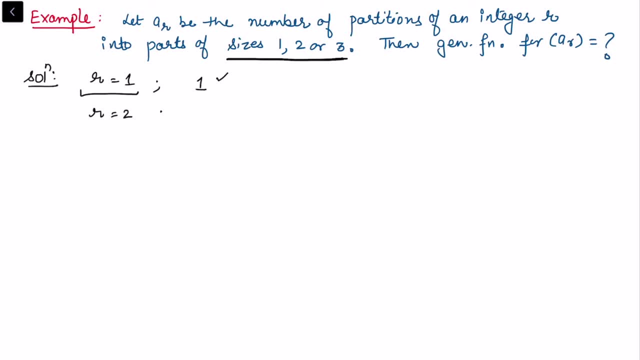 of 1 as 1. if r is equal to 2, there are two relevant partition, which is 1 plus r equal, and then we can take 2. so this is allowed if r is equal to 3, in this case we can definitely take 1. 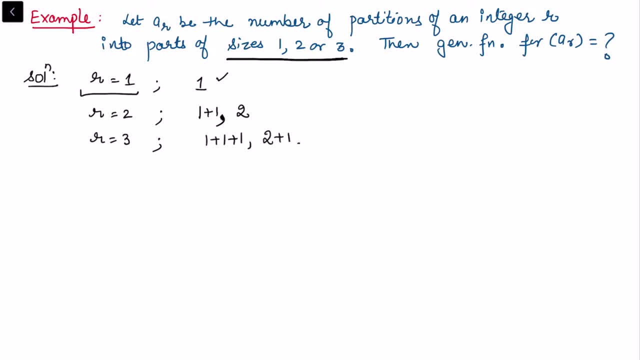 plus 1 plus 1, and then for 3 we can take 2 plus 1. we can also take 3, because 3 size is allowed if r is equal to 4. now in this case we can consider 1 plus 1 plus 1 plus 1, one partition. 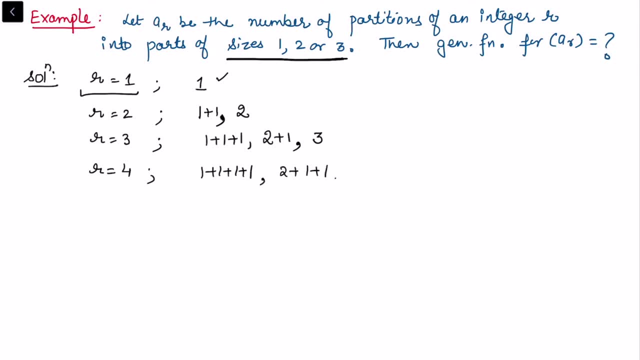 is this allowed? then we can consider 2 plus 1 plus 1. this is also allowed. 2 plus 2 is also allowed. we can also consider 3 plus 1, but 4. this is not allowed. this is not allowed. but earlier we have. 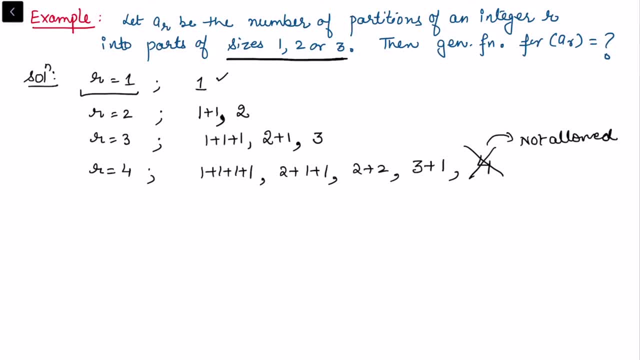 seen that 4 is a relevant partition, for n is equal to 4. now, 4 is not allowed because the sizes are only 1, 2 or 3. so now from here, we have an understanding that you can write a partition for any larger number, but the only condition is that we have to use the sizes 1, 2 and 3 only. 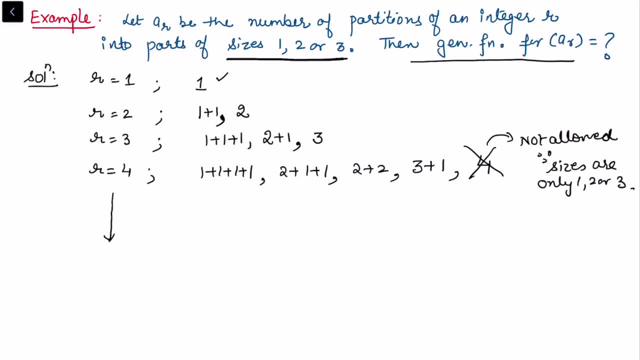 so now i want to know what is the generating function for this type of the partition here. if i write this in the notation so we can say: a1- this is equal to 1, a2- this is equal to 2, the coefficient of x square is 2, and that coefficient of x square is the number of partition of an. 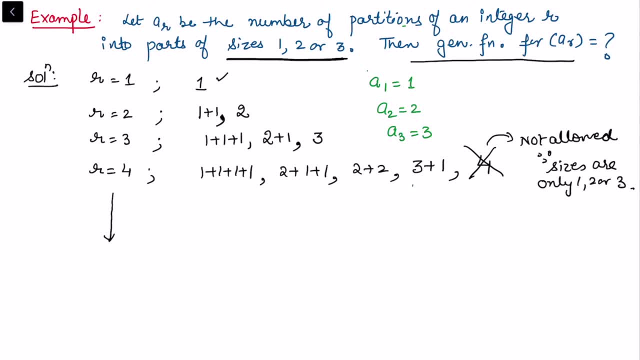 integer r, a3, this is 3 and here a4 is 4, not 5. so now in terms of generating function. so we recall what was the generating function. generating function for the sequence ar, so we can say generating function for ar. so this is a sequence, is summation of ar x to the power r, r goes from. 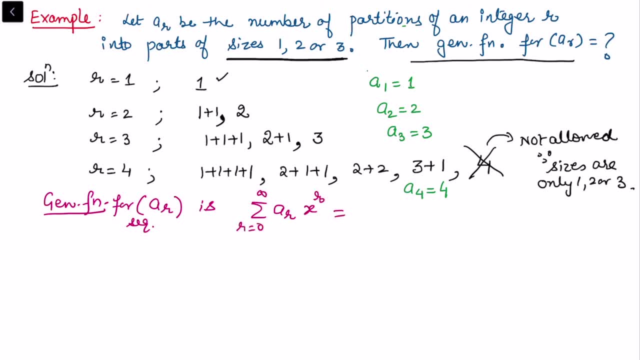 0 to infinity. and if i just open this summation sign, i will get it as a naught plus a1, x raised to power 1, plus a2 x square plus on up till ar x raised to power 1. so now, if i write this in the 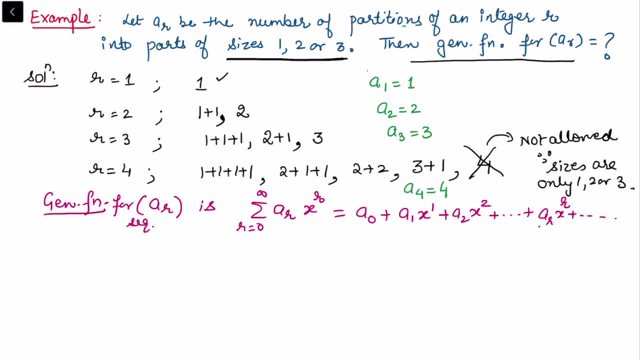 r plus on. so we are interested in knowing what is ar now. what is ar? ar is given to us, as in the problem, the number of partition of an integer r into the part size. so here here, ar given to us in the problem, this is the number of partitions of an integer r into parts of size. so we have 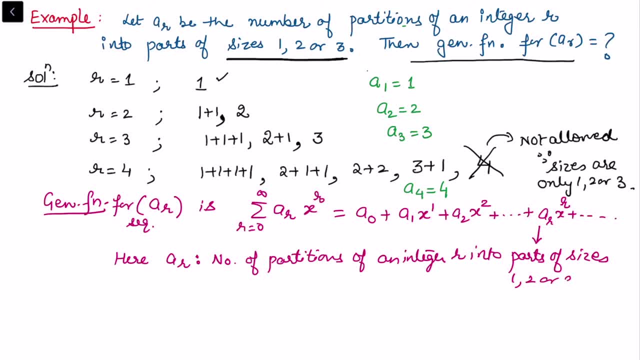 not mentioned how many parts that can go in any part, but the part sizes are mentioned: one, two or three and from the from this examples that we have verified, what we have verified, we have seen. so what we have verified, we have seen a naught, by default, this is one. a naught is actually the. 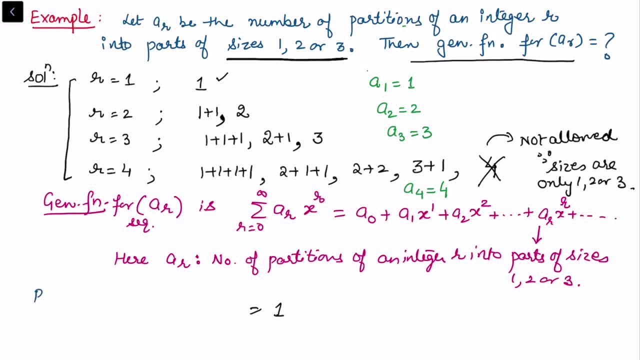 coefficient of x to the power zero. so we can note by convention: by convention partition of zero is considered as one, so we can always consider that as one and then a one. a one is a coefficient of x to the power one and we have seen one has. 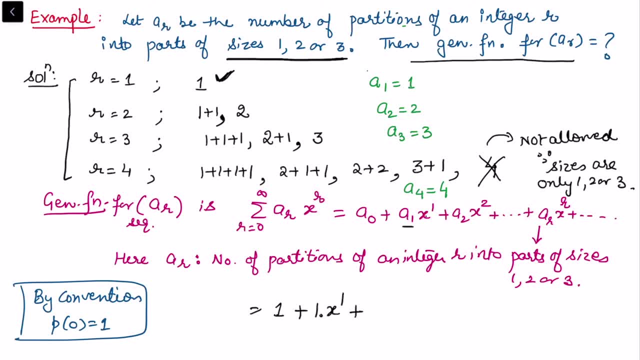 only one partition, so this is one into x to the power one. and for a two we have calculated a two is two, so there are two partition which are relevant to this condition, the coefficient of x- three, so there are three x cube and plus, so on, so on, and we can note down: this is the generating. 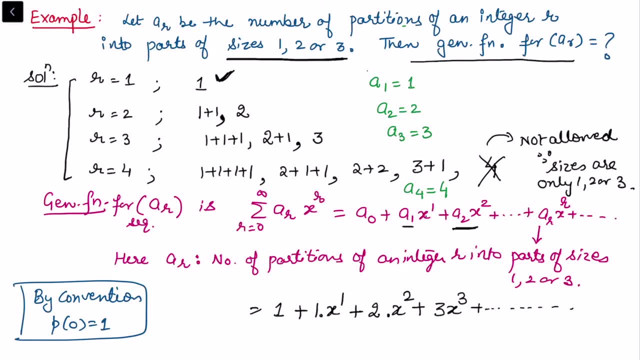 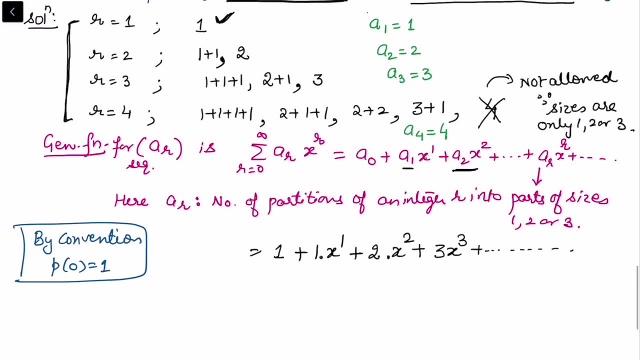 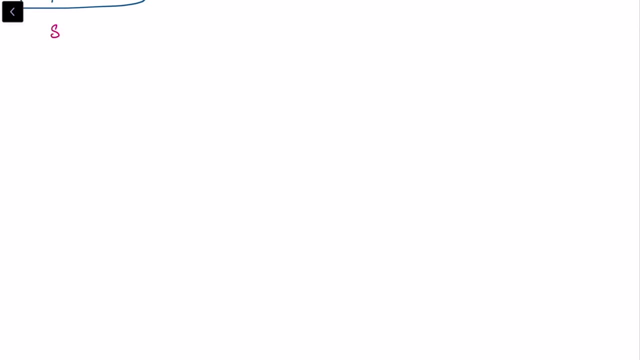 function. but now, how do we generate this? this is a few examples that i've listed, but if, in general, you want to understand how we have generated, so to know the other way around for the generating function, as we did in my last video, we can see the sizes are given to us as one, two. 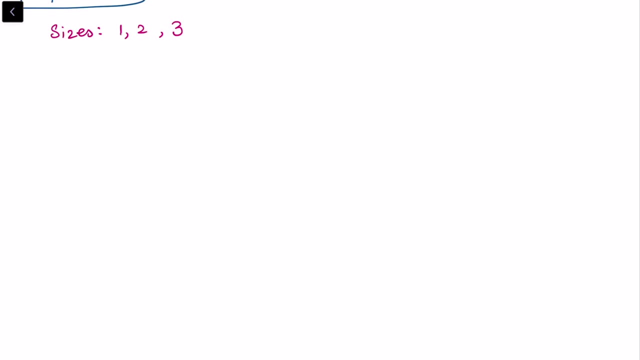 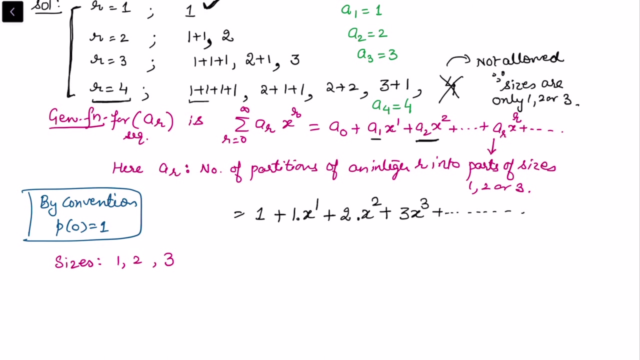 and three. so these are the three different sizes which can repeat any number of times. what do i mean by repetition? so we have seen, when we have considered r equal to four, one is repeating four times. so a part size can repeat as many as number of time. 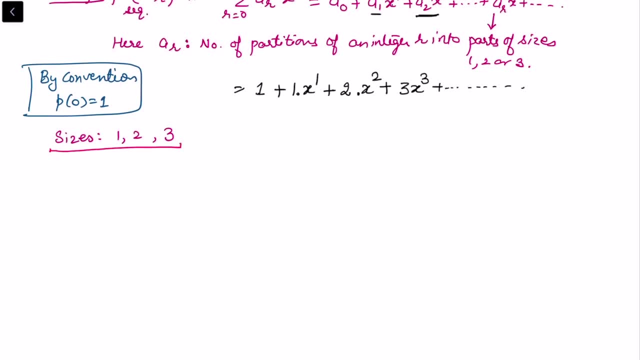 but the distinct parts that we are using also so. but the part sizes available with this is one, two and three. now, correspondingly, we write the generating function as first we will write corresponding to the size one, and then we will have the corresponding to size two, and then we 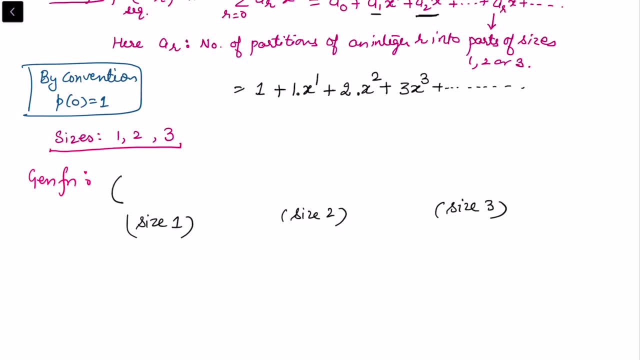 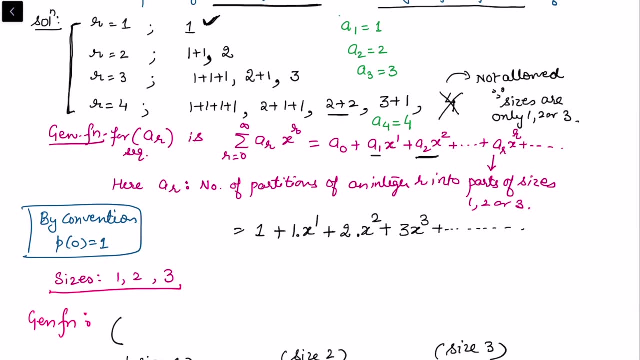 will have the corresponding to size three. now size one may appear or it may not appear. so for example: again we go back and we look at here the partition for r, equal to four. you can see that there is no part. one is used, size one is not used, two plus two. so here we have only used size. 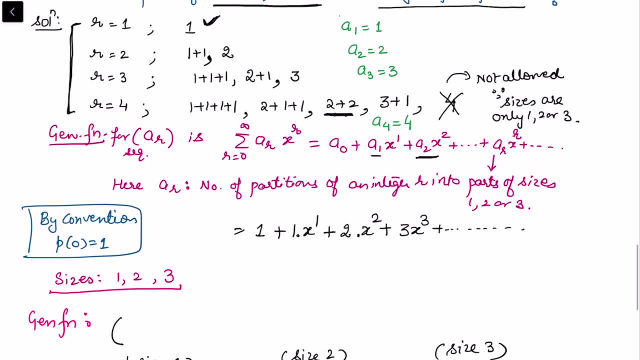 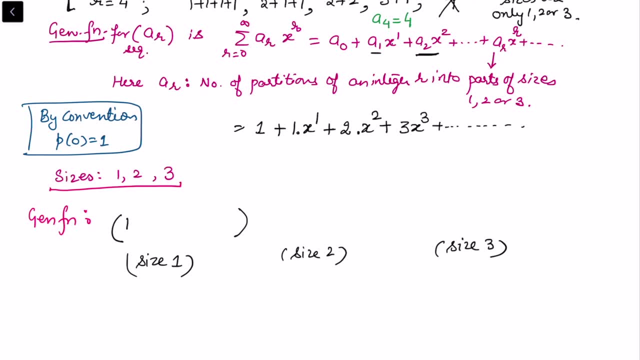 two, one and three are not allowed. so this means when we consider a generating function, size one may appear or it may not appear. if it is not appearing, then this is one. one means x to the power zero, x to the power one plus x square. so here we are considering size one appearing many. 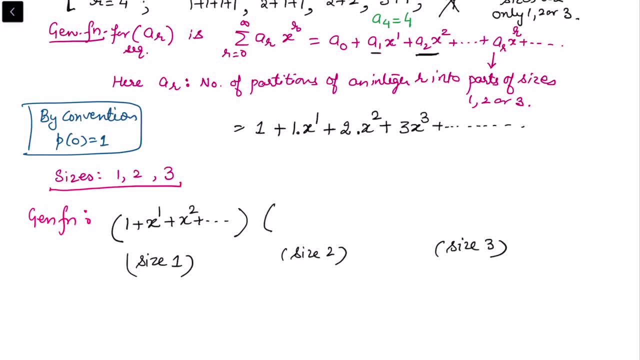 times. okay, and here we are saying size two. size two means we will start from x square. okay, let me to rewrite this generating function in a more specific way. we can say size one appear zero times. we can say size one appear one time. we can say size one appear two times and we continue this one. we can say the size two x square. so we are. 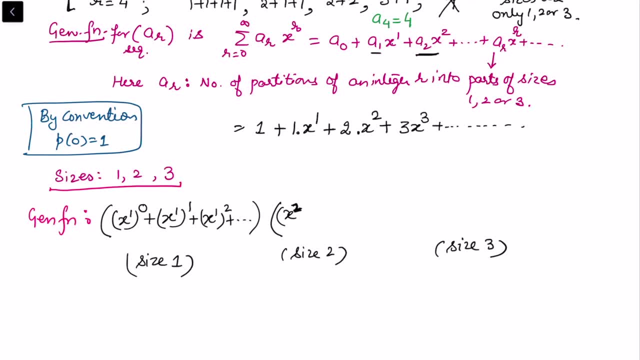 talking about a partition of two number, and then it's repetition: it is appearing zero time. partition of two appearing two times. this means actually it is giving a partition of four and plus so on. it can appear as many as number times. then partition of three appearing zero times, plus partition of 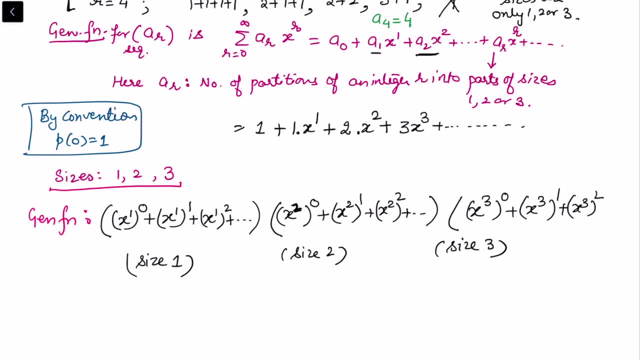 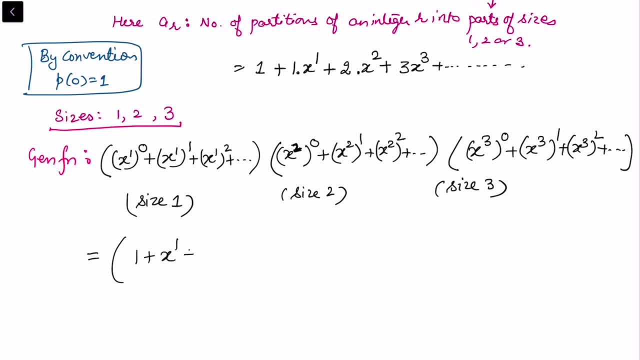 three appearing one time, partition of three appearing two time and so on, which we can further write it as one plus x to the power one plus x, square plus so on. this we can write one plus x, square plus x to the power four plus so on, and this one we can write one plus x cube, plus x to the power six plus so on, and if I 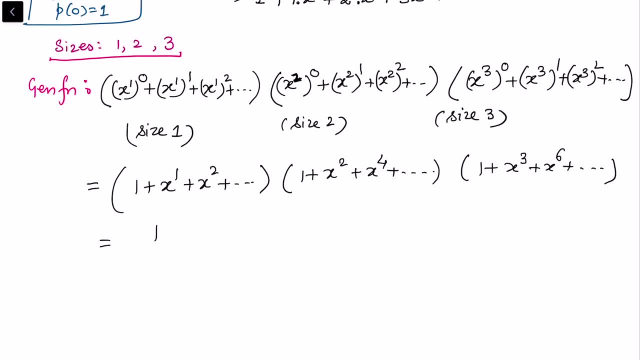 look at in this generating function you can see that this is like a GP and here the common ratio is x, so it is one over one minus x. in the second term you can see the common term common ratio is x square. so this will give me one minus x square. and in the third term you can see that this will. 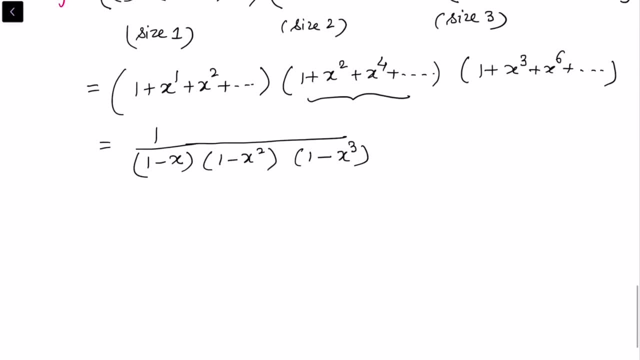 be one minus x cube, so this becomes the generating function. now, if I want to understand the generating function, or any terms that may appear from here, suppose if I look at the example, let the coefficient- we have already seen the coefficient of x Cube. this is three in the expansion. we have already. 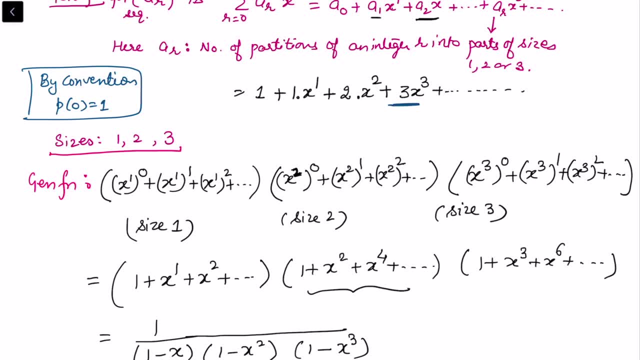 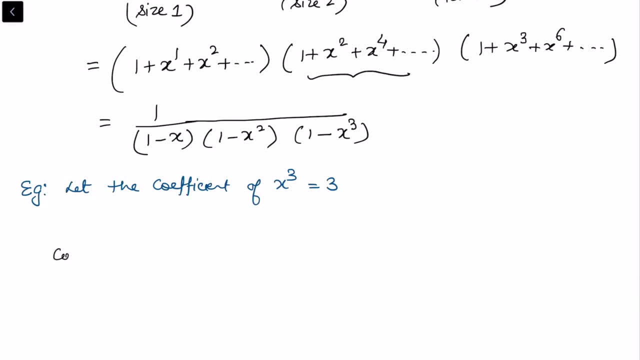 seen in the previous expansion. you can see the coefficient of x 3 is equal to 3.. suppose I want to read directly from here how do I read the coefficients of a particular term? and here, if I want to read the coefficient of x cube in the given generating function, which was 3, we know we use three sizes: size 1, size 2. 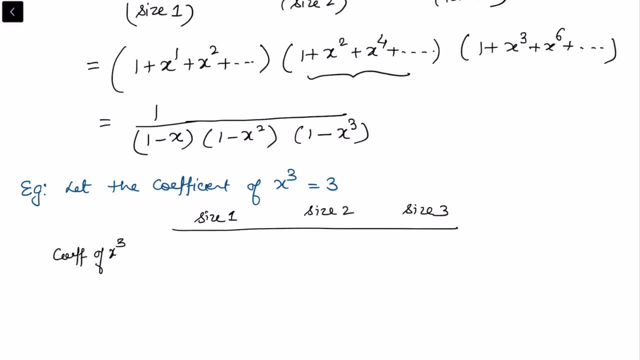 and we use the size 3. now we know the size 1 is due to this term, size 2 is due to this term and size 3 is due to this term. so if i look in this expansion, so this is due to size 1. if i look at, 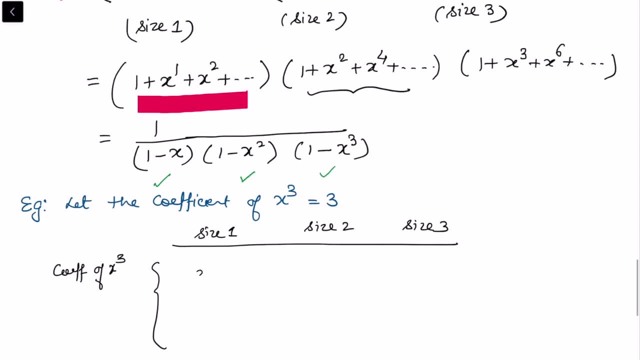 here corresponding to this. one suppose, if i take x to the power 0, and here also i take x to the power 0, and in the last term if i take x cube, so this will give me a partition of 3 which is equal to 3. so this is the relevant partition n, and here i am writing the relevant partition. so what i did. 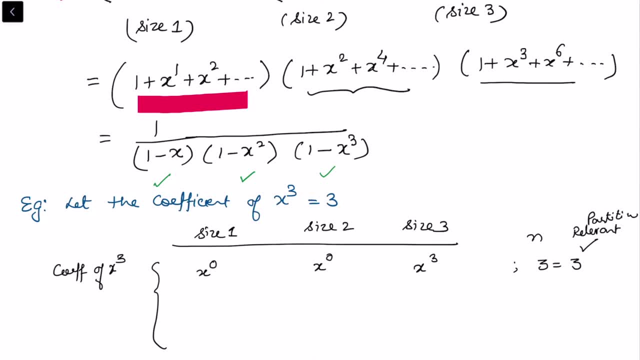 when i looked at these generating function, individual term. if you multiply this constant, this one, with this one, and here you multiply with x cube, that's the term when i'm taking x 0, here also x 0 and here i'm taking x cube. so if you add these coefficient, we get that. we are going to get a partition of 3. this is going to. 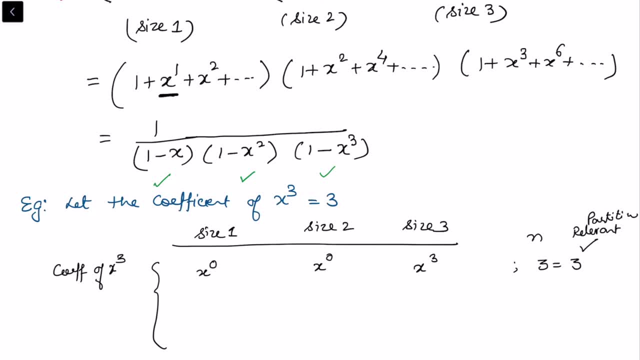 give us the coefficient x cube. now take x to the power 1 from here, take x square from here. when you multiply these two, then also the total power will be x cube and in this case we just need x to the power 0 from here. so we will have another possibility: x 1, x square, x 0 and in this case 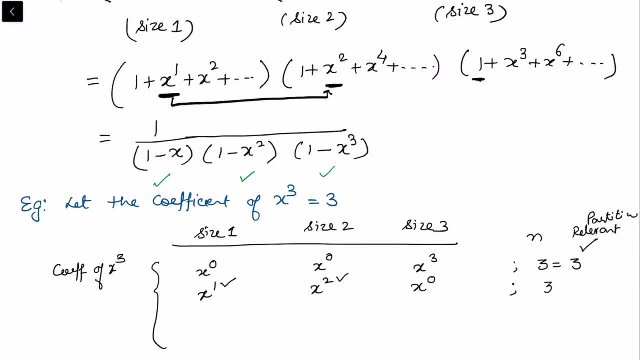 you can read the power: this is 1 and in this case, you can read the power: this is 1 and in this case, you can read the power: this is 1 plus 2, so this is a partition of 3, but which is due to 1 plus 2, so we can even read the. 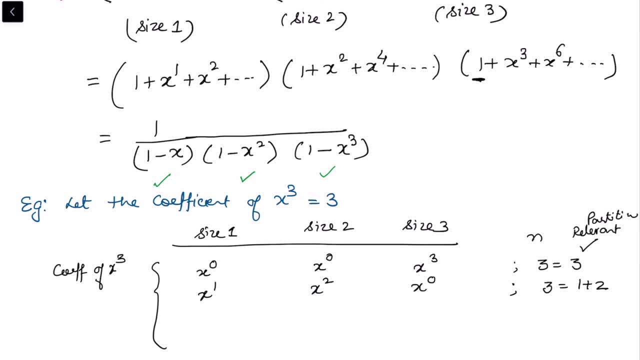 corresponding relevant partition. now, on: the same way, if i take x, if i take x cube from the first bracket, so that's x cube will be here and this x cube if i multiply by the constant and this constant, then also i will get x cube. here it is x 0, here also it is x 0, and in this case now, 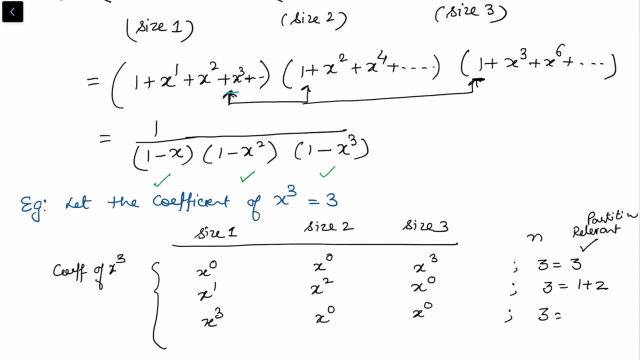 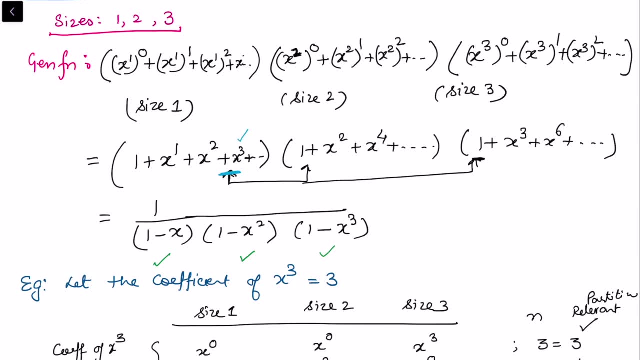 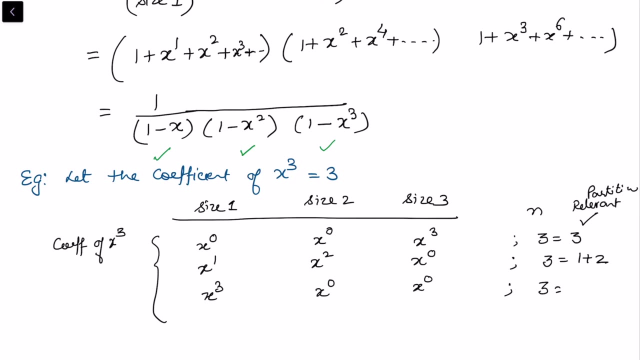 once it is in this particular bracket. we have taken it from the first bracket. this means 1 is repeating 3 times. it must have been taken from this case x, 1 appearing 3 times. so this is how we have taken. so means that we write here: we write here 1 plus 1 plus 1 because it is using the size. 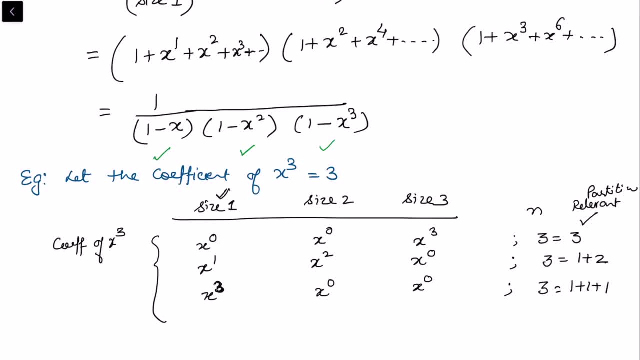 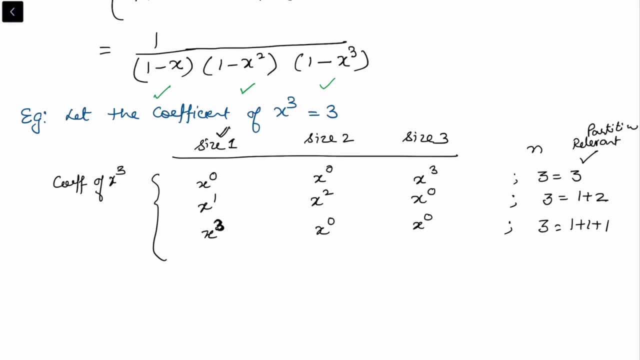 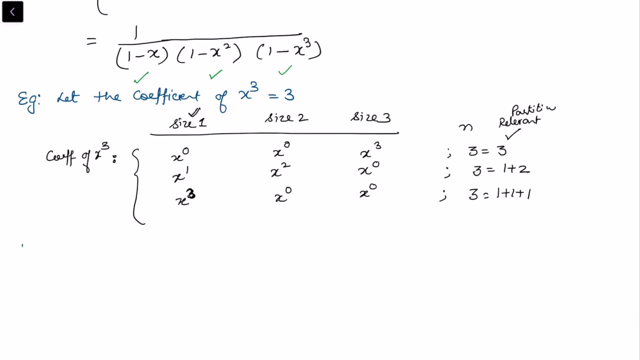 1. so size 1 is appearing 3 times. so this is the way we read the corresponding relevant partition, and we can also read the corresponding coefficients of the relevant size. now let's say i want to write one more term here, and here i want to write the coefficient of x to the power 4. 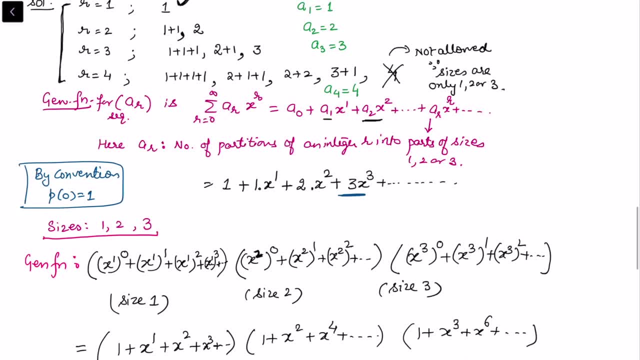 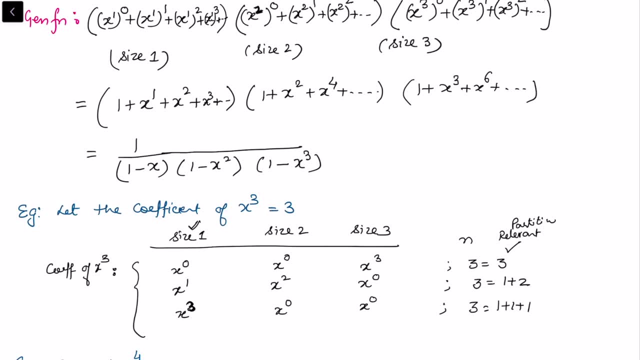 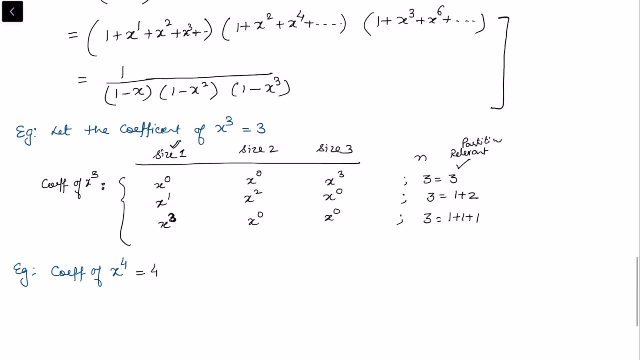 so we just have verified in the previous case, the coefficient of x to the power 4 is 4 and i want to extract these four coefficient from this expression, from either this expression or from this expression. so now, if i want to write the coefficient of x to the power 4, these, this was 4, let's extract. 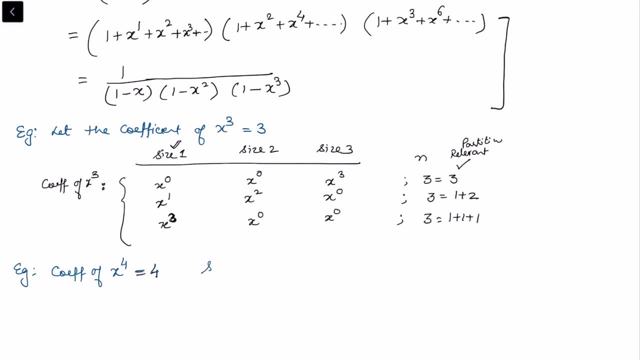 again from the sizes. so this will be size 1 here, it will be size 2 here, this will be size 3, and if i just look at here, once we take x to the power 0 here, then if i take x so we can write it. 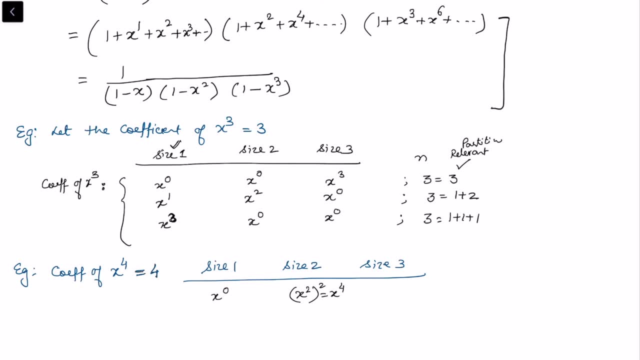 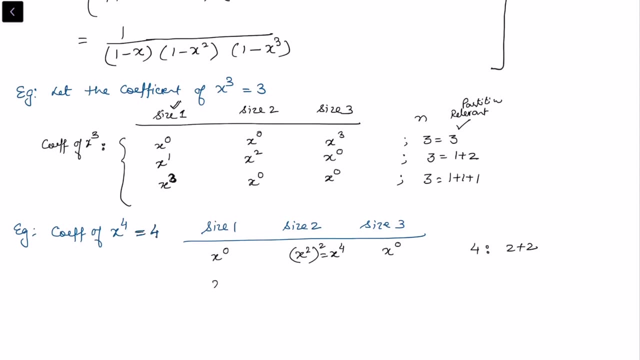 x square square. this means this is x to the power 4, and here i'm taking x 0. that means the relevant number is 4. 2 is repeating 2 times. then we can take x to the power 1. here let me to take. 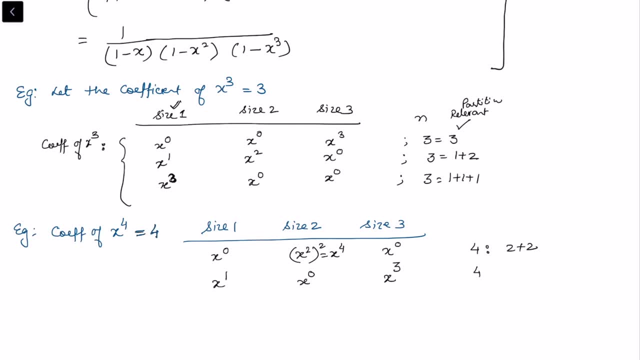 x 0 here and here i will take 3. this will lead to a partition of 4 with 1 plus 3 as a part. then i can take x square here and i can take x squared here, x squared appearing one time- because when you say size 2, this means actually the variable is x squared now. 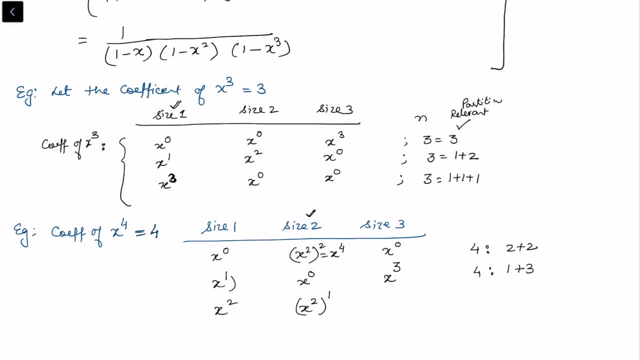 that variable can repeat as many as number of time. here x raised to the power 1, repeating one time. here x raised to the power 1, repeating 2 times. and that nowadays we indicate that one of the endpoint is zero. so we say that the now that means inside the coding transaction. 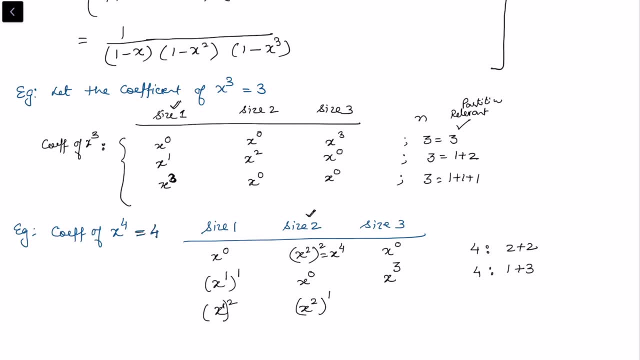 is 1, so the following is the Truman equation as wave 1, commune 1, leaf 1 length 1 Koch, Brady, Keller times, and that is how it was x square, in this case x, 3 appearing 0 times. so or you can simply write x to the power 0, and so in this case this will be 4 appearing due to this factor and this. 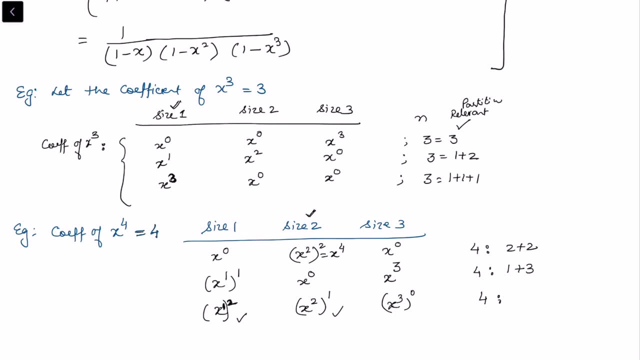 factor 1 is repeating 2 times and 2 is repeating 1 time, so this will be 1 plus 1 plus 2. 1 is repeating 2 time and 2 is appearing 1 time. now we'll write all possible combinations of this. 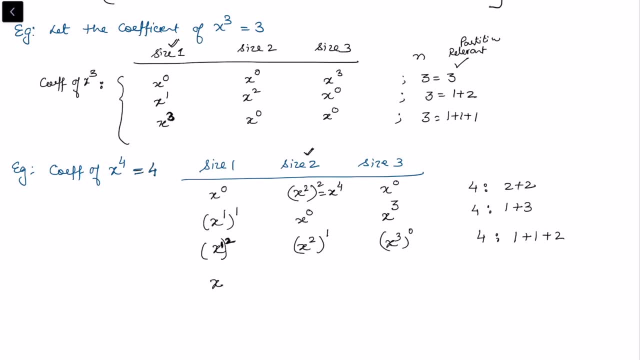 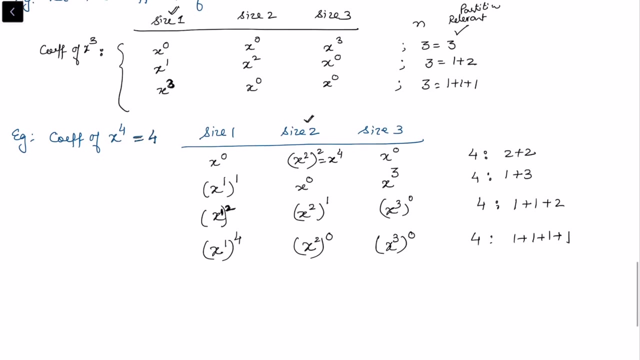 one and we'll see that this is coming correctly. and then now you can have 1 repeating 4 times, you can have x square coming 0 time, you can have x 3 coming 0 time, and so in this case we are talking about 1 plus 1 plus 1 plus 1. now, in any other combination we will not be able to generate. 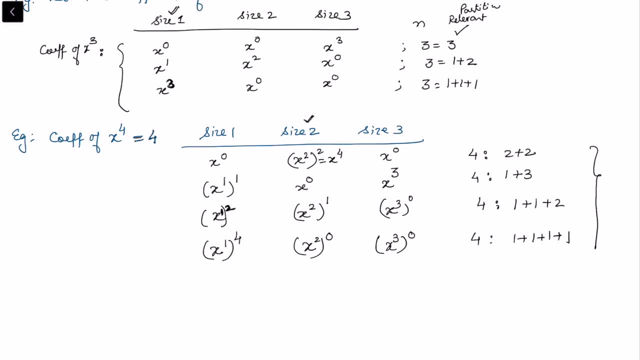 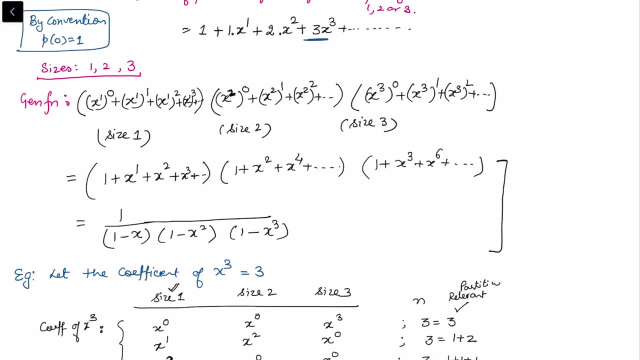 any other partition of 4, either this number will increase or the this number, n, will start decreasing. so we know that this, by defining the sizes, size 1 and size 2- we will be able to generate any other partition of 4, and so in this case we: 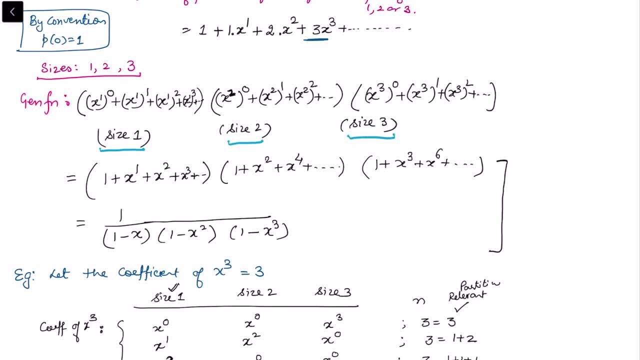 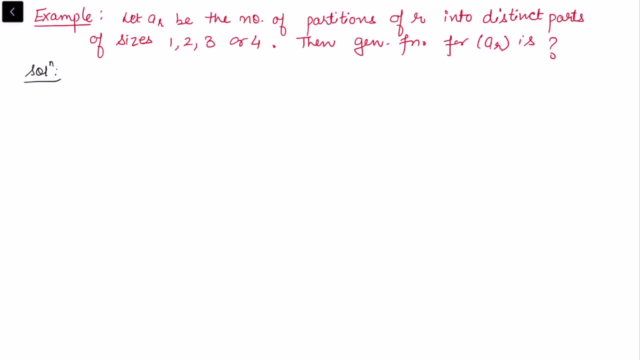 can construct this as a generating function for partition, and here the number of parts are not restricted, rather the size of the part is fixed, and we have used size 1, 2 and 3. now in this example we want to find again the generating function for ar, where ar be the number of partition of r. 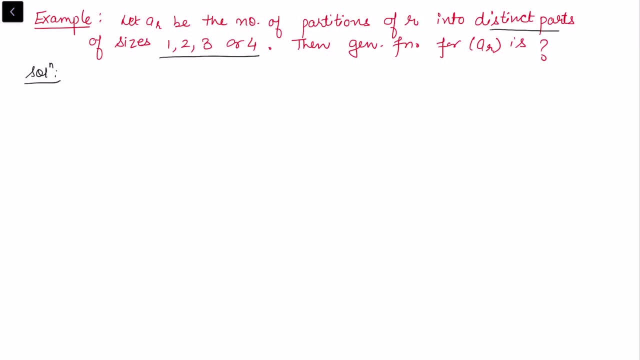 into distinct parts of sizes: 1, 2, 3 or 4. so what do i mean by distinct parts of sizes? so sizes are defined first of all, and these sizes we can use- 1, 2, 3 or 4- and then we also said that the parts are. 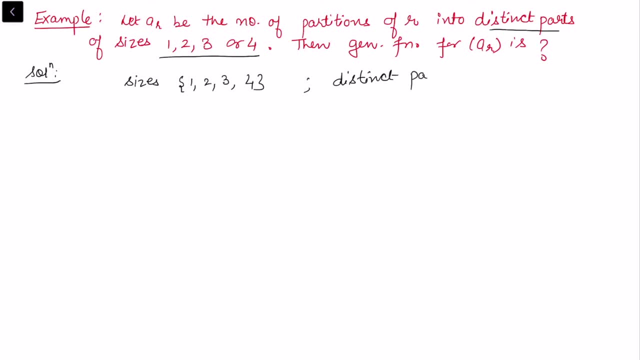 distinct. so that means, a part of a particular size cannot repeat. so for example: when i take n is equal to 1, then 1 is allowed. when i take n is equal to 2, 2 is allowed, 1 plus 1. this particular partition is not allowed, because here the parts is repeating. okay, because 1 as a part repeats, but we want part. 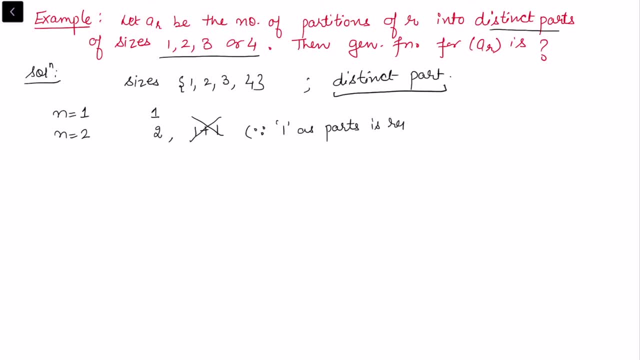 to be distinct part. part is repeating, so this is not allowed now. similarly, when i take n is equal to 3, so in this case i can take 3, 2 plus 1, and then we cannot take 1 plus 1 plus 1. this is not. 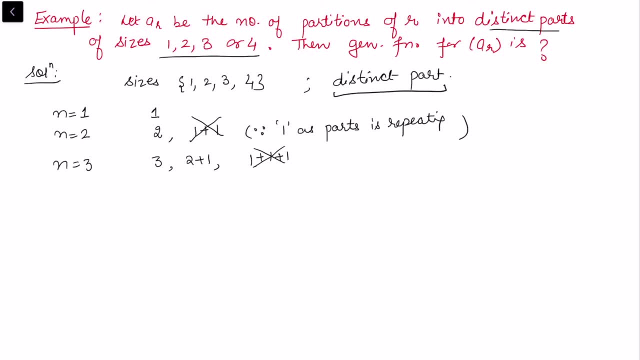 allowed, because here of course it is repeating, and in this case the coefficient, when i construct a sequence here, a1, this is equal to 1. in this case a2, this is also 1. there is only one relevant partition in this case. a3, this is 2, and this is also 1, there is only one relevant partition in this case a3, this is 2. 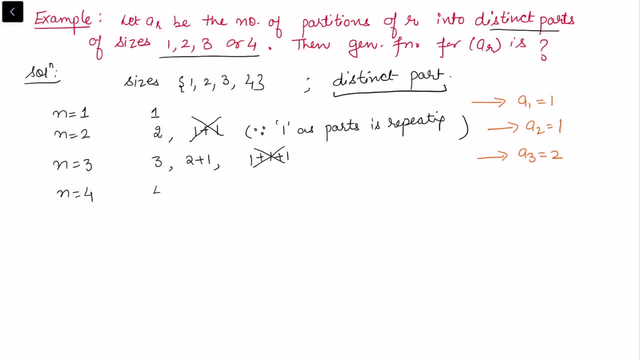 and if i just increase n is equal to 4. 4 is allowed because the part size 4 is allowed. then we can take 3 plus 1. we cannot take 2 plus 2. this is not allowed. we cannot take 2 plus 1 plus. 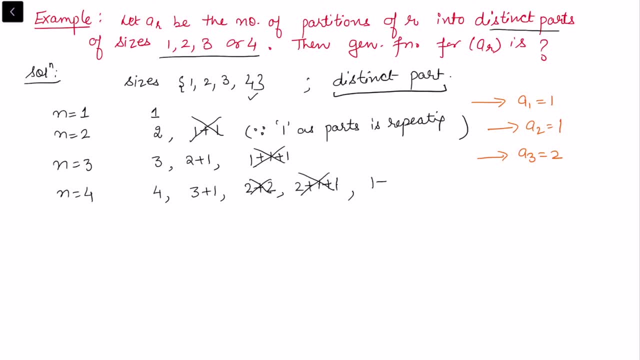 1, because 1 plus 1 is repeating. this is not allowed. and then we also cannot take 1 plus 1 plus 1. this is also not allowed. so in this case also the coefficient a4. this is equal to 2, so you can. 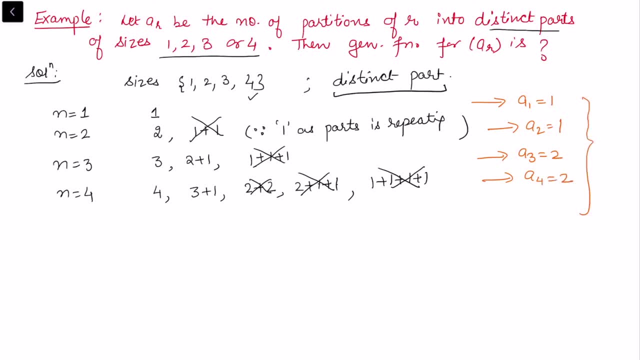 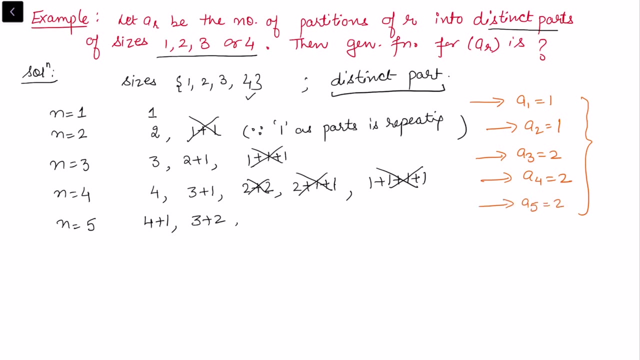 see how this number get changed. depending upon various restriction on the partition, the number gets changed and so you can find: for n is equal to 5. in this case we can have 4 plus 1. we can have 3 plus 2. these are the only two possible relevant partition for 5. now i want to know what is the 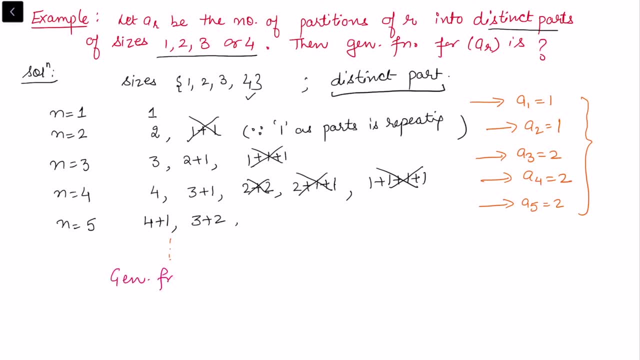 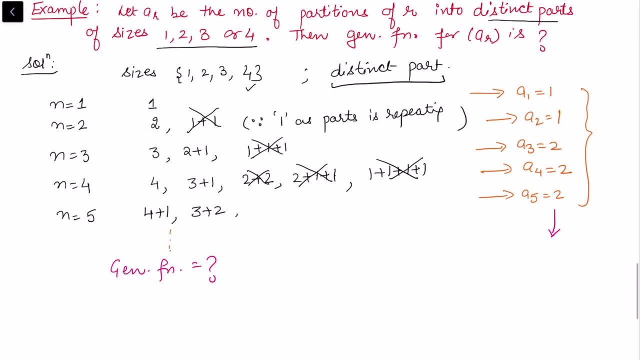 generating function corresponding to this one? what is the generating function which generate these numbers as a sequence? and so for this one, we know that part will not repeat. okay, it's, it will come only once or it may not come, like for example in this 3 plus 2 part. size 1 is allowed. 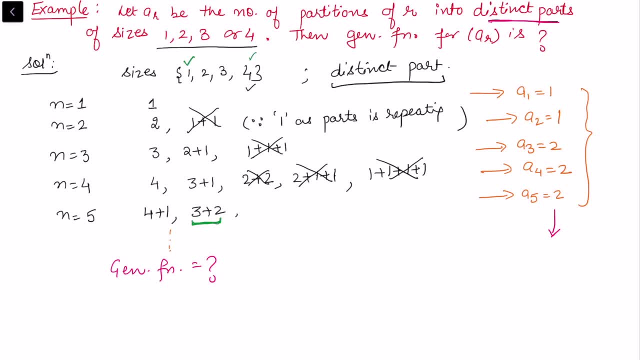 part size 4 is allowed, but they are not coming. so the only restriction is the part size may appear or it may not appear, but it will appear only maximum. it will appear once, so that it maintain the distinct condition. so what will be the generating function here? there are four part. 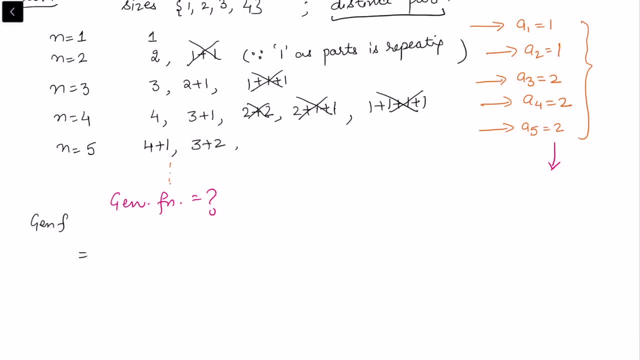 sizes. so we will write the generating function for the sequence ar is for the part size 1, and then for the part size 2, and then for the part size 3 and for the part size 4 now, if 1 is not repeating. so this is: x raised power: 1 not coming. x raised power: 1 coming. 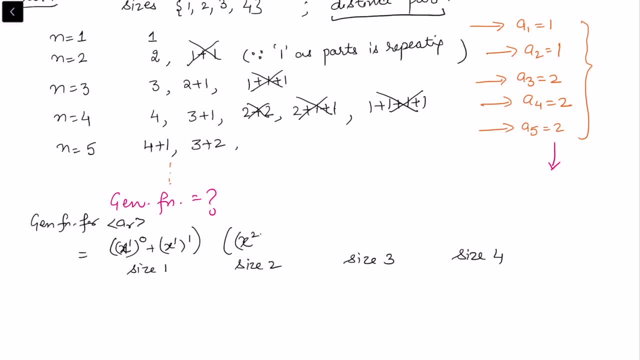 once that's allowed: x square not coming, x square coming once. x cube not coming and x cube coming. similarly, x to the power 4 not coming and x to the power 4 coming once that's the generating function. so in my previous example we did not had the distinct condition, so this sequence was: 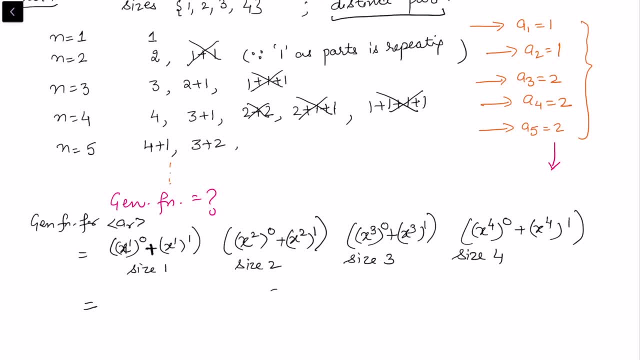 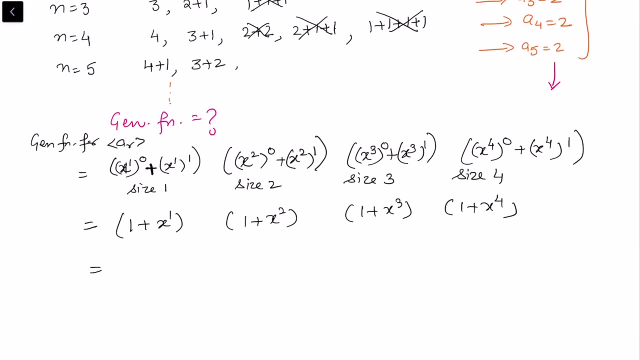 actually going plus, plus, plus infinity in every parenthesis, but now we have to bound this. so this is 1 plus x to the power 1, then we got 1 plus x square, then we got 1 plus x cube, and we got 1 plus x to the power 4. now, if we just multiply this term, we can see that 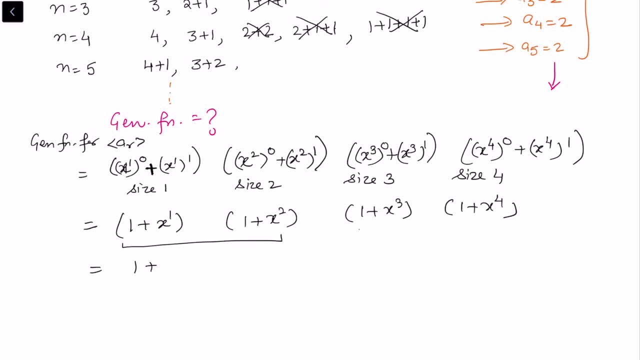 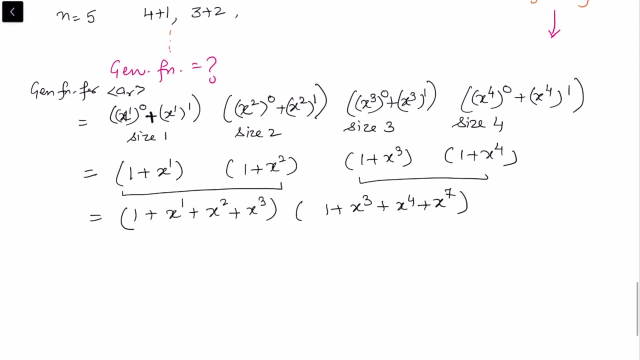 we will have 1 plus. so let me to first multiply these two and then we look at the sequence: x to the power 1, then we got x square, then we got x cube, and then if we, if I multiply this one, x cube, x 4, and then we have x to the power 7, and if I just re-multiply these two term again, so we 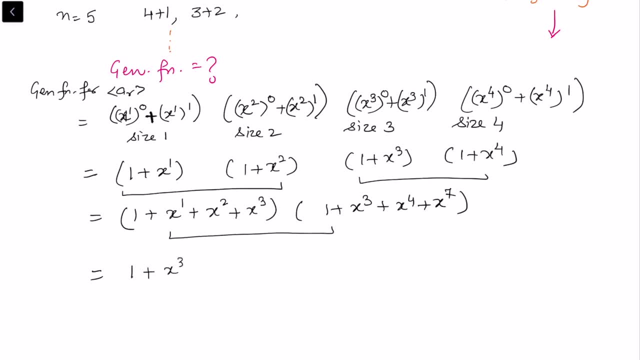 notice that we will have 1 plus x cube plus x 4 plus x to the power 7. so when I multiply 1 with the next parenthesis, then we get x square. and then if I multiply x to the power 1 with the next parenthesis, this is how I will get the terms. and then when I multiply x square, then we got 5 x to. 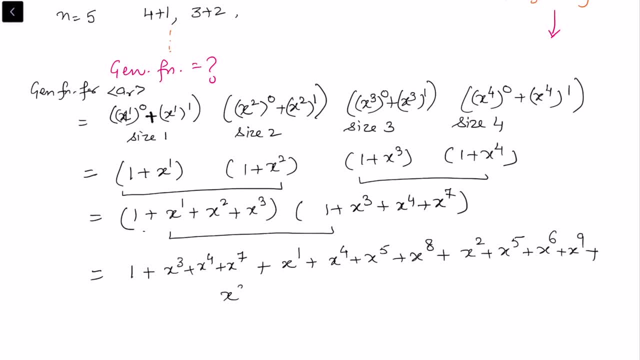 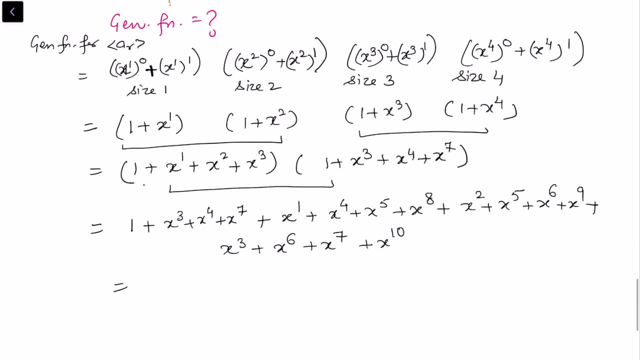 the power 6 plus x to the power 9, and if I just multiply the last term, we got 6, x to the power 7 and x to the power 10. that is the sequence. and here, if I just rearrange the terms in the increasing 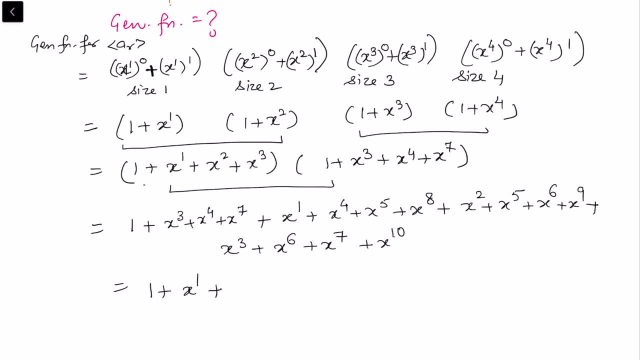 order. so we have 1 plus x to the power 1 and then we will have x square and you notice that there are two term corresponding to x 3, so this is 2 times x cube. then similarly, for x 4, we have two terms. so 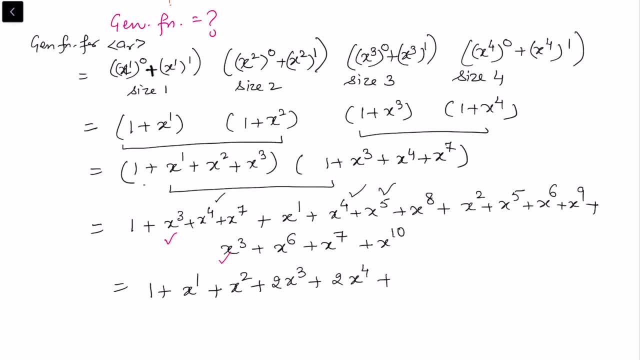 this is 2 times x, 4 for x to the power 5. also we have two terms: 2 times x to the power, 5. for 6 also, we have 2, 2 times x to the power, 6 for 7 also, we got 2 times x to the power 7 plus x to the power. 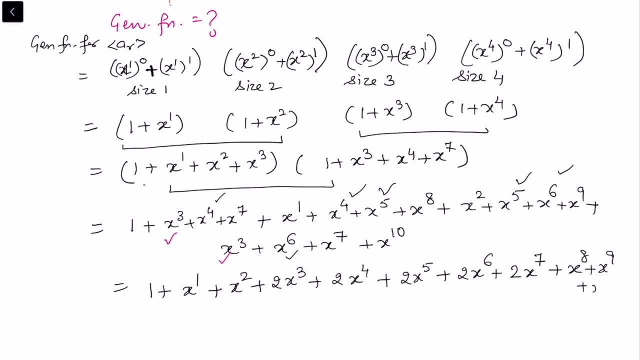 8, plus x to the power 9 and plus x to the power 10. now if, if I look at carefully here, the coefficient of x cube is 2, coefficient of x, 4 is 2, x 5 is 2, x square is 1, x raised to the power 1 is 1 and this is the.